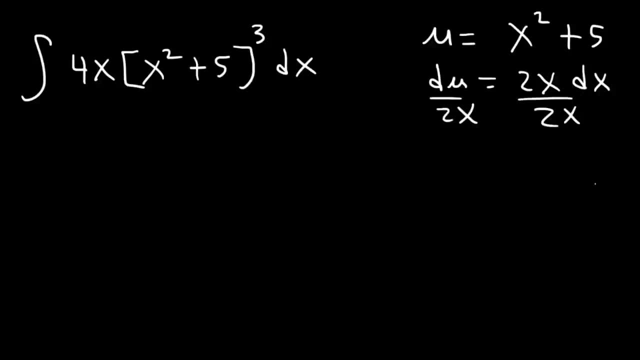 divide both sides by 2x. dx is equal to du divided by 2x. Now what you need to do is replace this with u and replace the dx with du over 2x, and it will all work out. So let's go ahead. 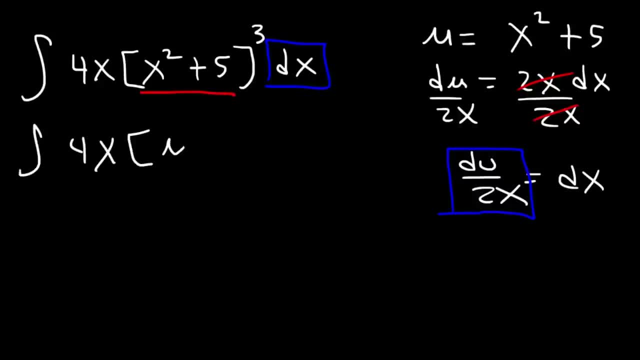 and do that. So we have 4x and then u raised to the third power and then du divided by 2x. So here we can cancel x. 4x divided by 2x is 2.. So it's 2 times. 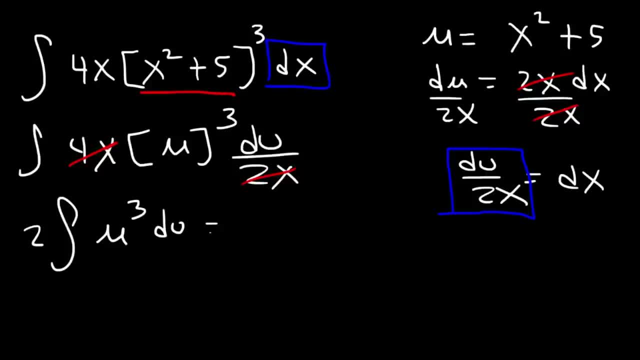 the antiderivative of u to the third. Using the power rule, it's going to be 2 times 2x. u to the fourth over 4 plus c. Now 2 over 4 is 1 half, So it's 1 half u to the 4th. 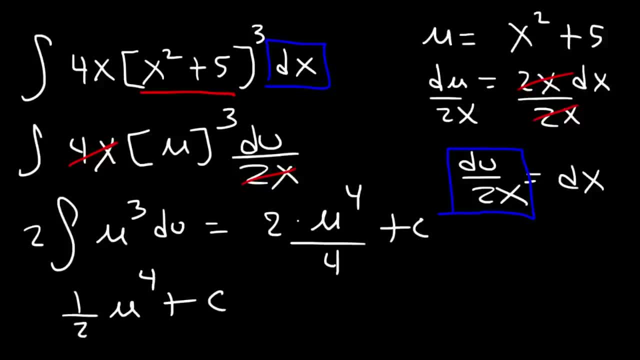 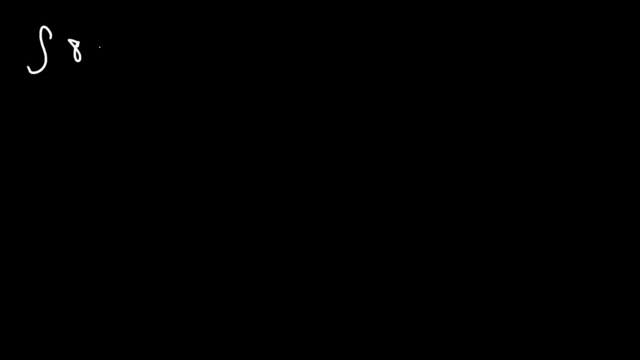 plus c. The last thing you need to do is replace u with what it equals, and that's x squared plus 5.. So this is the answer. Let's try another one. Here is another problem. Go ahead and find the integration of 8 cos 4xdx. 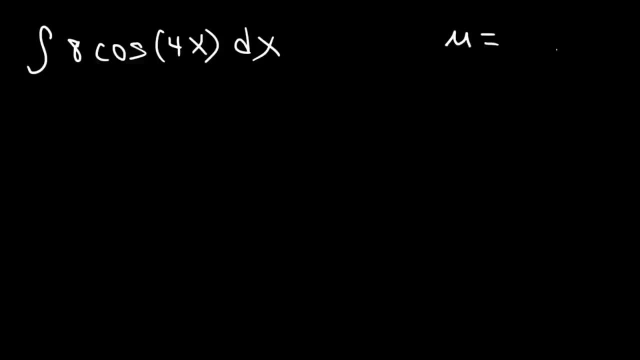 So what should we make u equal to? We need to make u equal to 4x. du will equal 4dx, And if we divide by 4, du over 4 is dx. So let's replace 4x with u and let's replace dx with 4x. It's ú equals. 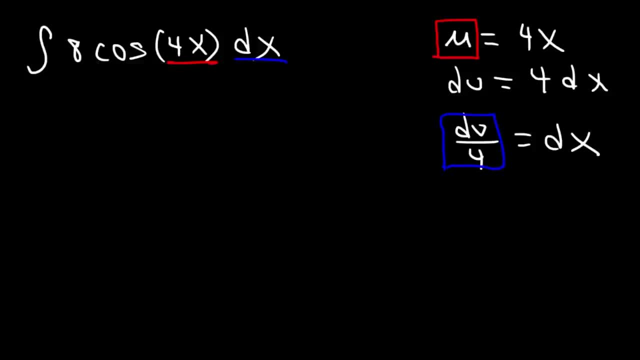 4dx du divided by 4.. So this is going to be 8 cosine of the u variable and replace dx with du over 4.. So now we can divide 8 by 4.. 8 divided by 4 is 2.. Now what is the? 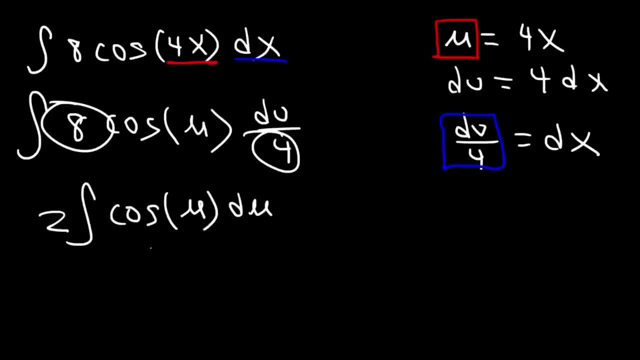 antiderivative of cosine. The antiderivative of cosine is sine, because the derivative of sine is cosine. So we have 2 sine u plus the constant of integration c. Now let's replace u with 4x, So the final answer is 2 sine 4x. 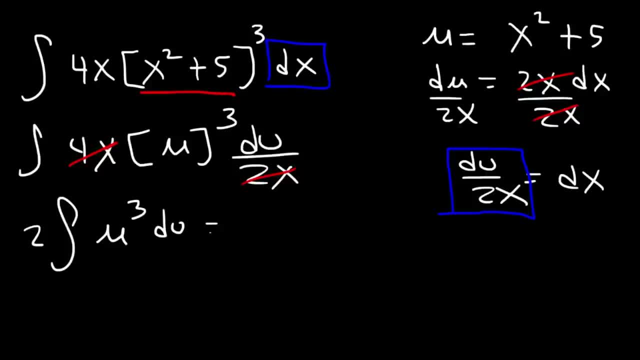 the antiderivative of u to the third. Using the power rule, it's going to be 2 times 2x. u to the fourth over 4 plus c. Now 2 over 4 is 1 half, So it's 1 half u to the 4th. 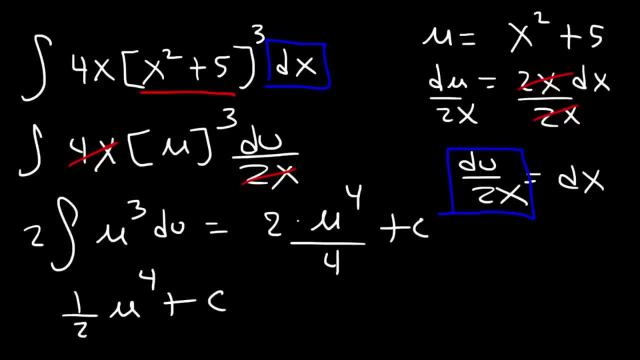 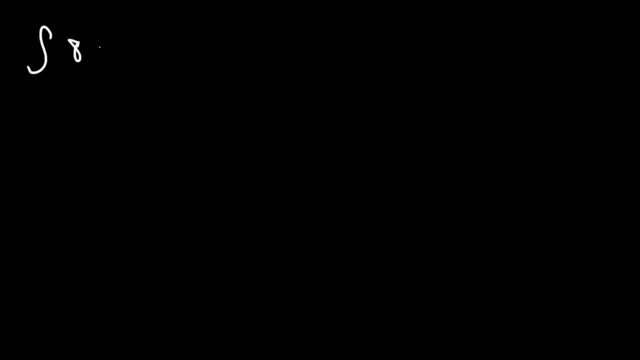 plus c. The last thing you need to do is replace u with what it equals, and that's x squared plus 5.. So this is the answer. Let's try another one. Let's try another problem. Go ahead and find the integration of 8 cosine 4x dx. 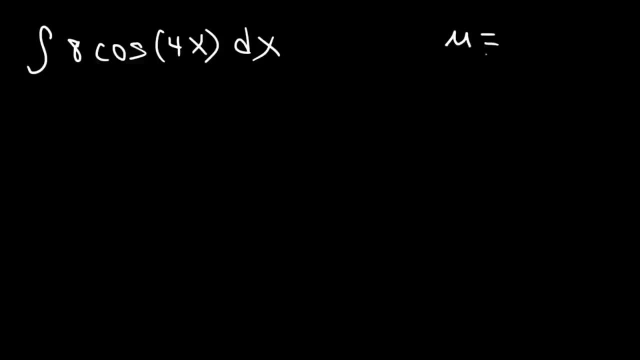 So what should we make u equal to? We need to make u equal to 4x. du will equal 4dx, And if we divide by 4, du over 4 is dx. So let's replace 4x with u and let's replace 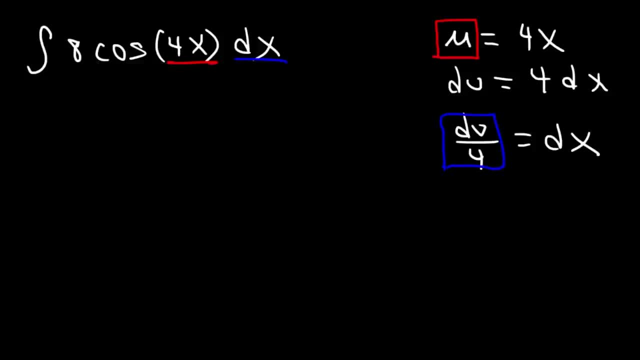 dx with 2x du divided by 4.. So this is going to be 8 cosine of the u variable and replace dx with du over 4.. So now we can divide 8 by 4.. 8 divided by 4 is 2.. Now what is the? 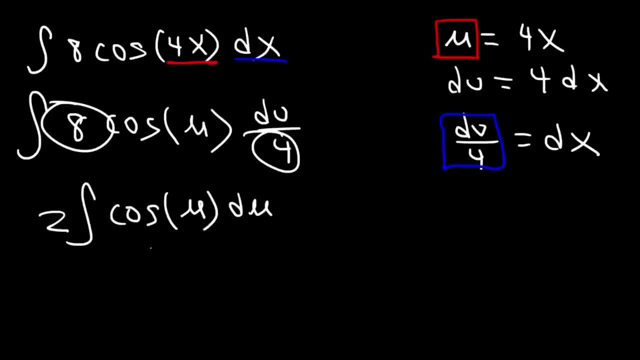 antiderivative of cosine. The antiderivative of cosine is sine, because the derivative of sine is cosine. So we have 2 sine u plus the constant of integration c. Now let's replace u with 4x, So the final answer is 2 sine 4x. 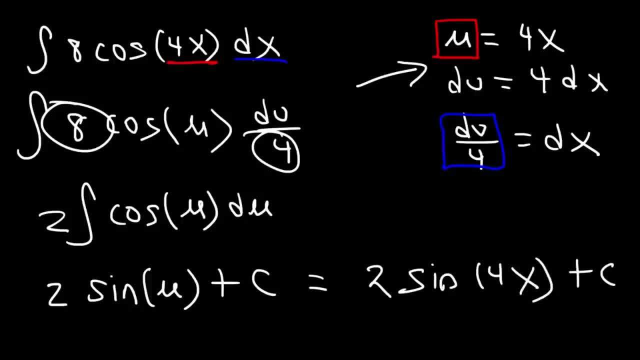 plus c. So hopefully you see a pattern emerging. when integrating by u substitution, The key is to identify what u and du is going to be. Once you figure that out, you just got to follow the process and it's not going to be that bad. So let's work on a few more examples so you can master this technique. Let's 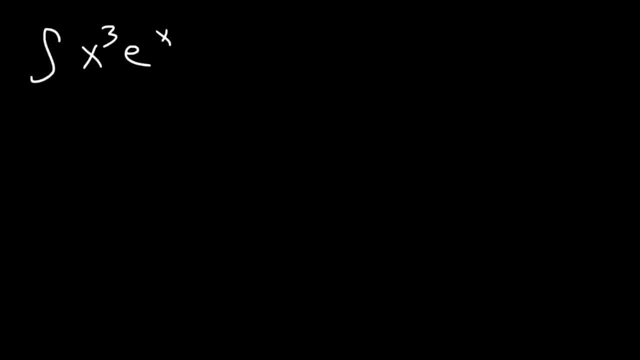 try: x cubed, e raised to the x to the fourth. So what should we make? u equal to x cubed or x to the fourth? If u is x to the third, du will be 3x squared and that will not completely get rid of x to the fourth. But if we make u equal to x to, 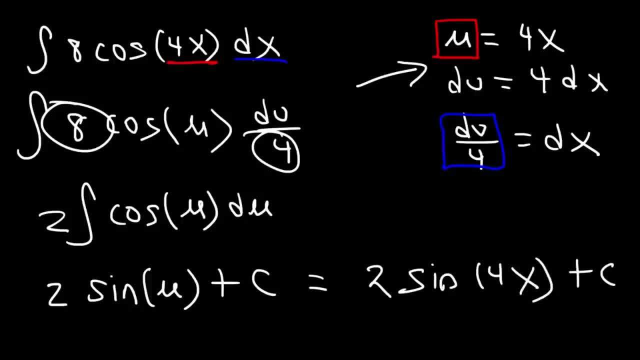 plus c. So hopefully you see a pattern emerging. when integrating by u substitution, The key is to identify what u and du is going to be. Once you figure that out, you just got to follow the process and it's not going to be that bad. So let's work on a few more examples so you can master this technique. Let's 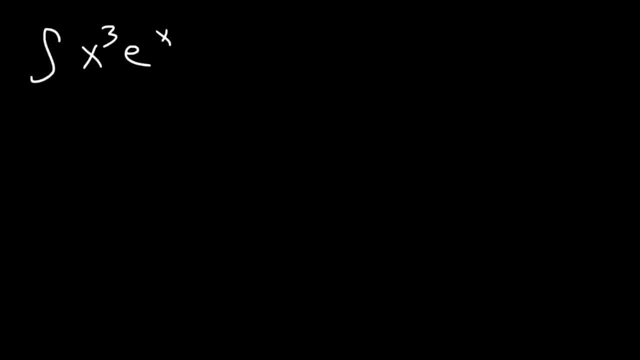 try: x cubed, e raised to the x to the fourth. So what should we make? u equal to x cubed or x to the fourth? If u is x to the third, du will be 3x squared and that will not completely get rid of x to the fourth. But if we make u equal to x to, 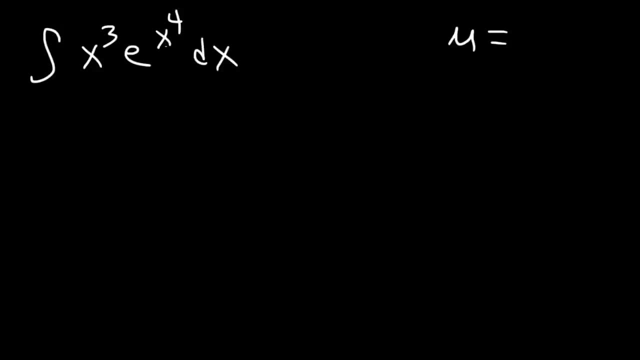 the fourth, du will be equal to 4x cubed, and that can get rid of the x cubed that we see here. So let's do that. Let's make u equal to x to the fourth. So du is going to be 4x cubed, dx, and then, as always, solve for. 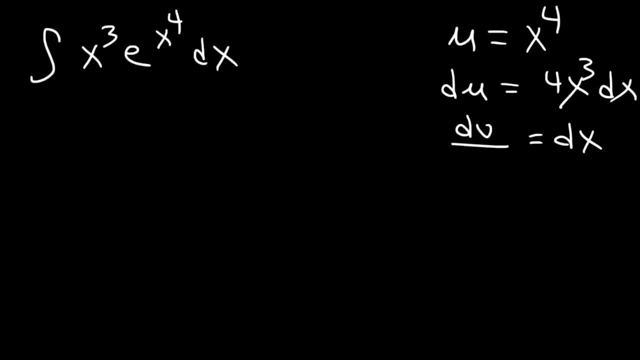 dx. If you don't do that, you can easily make some mistakes. so I recommend, in this step, isolate dx. It'll save you a lot of trouble later on. So du is going to be- I mean dx is going to be- du over 4x cubed. Now let's replace x to the fourth with. 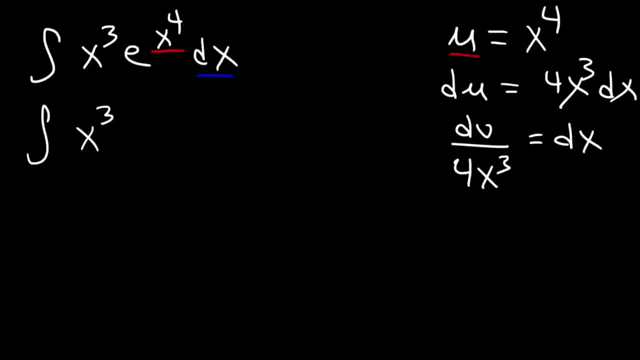 with u and let's replace dx with du over 4x cubed. So this is going to be e raised to the? u times: du over 4x cubed. So x cubed will cancel, which is good, and the 4 we can move it. 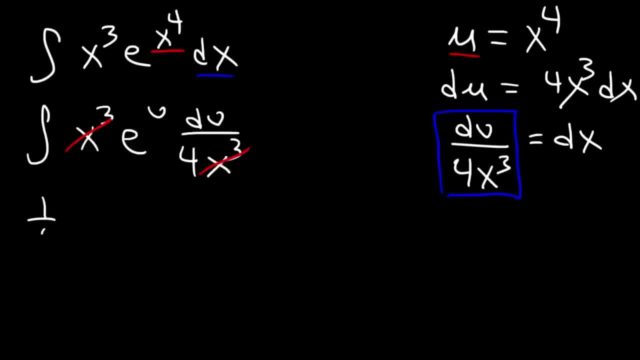 to the front Now, because it's in the bottom of the fraction, it's 1 over 4.. Now the antiderivative of e to the? u is simply e to the? u. So the final answer? well, not the final answer, but 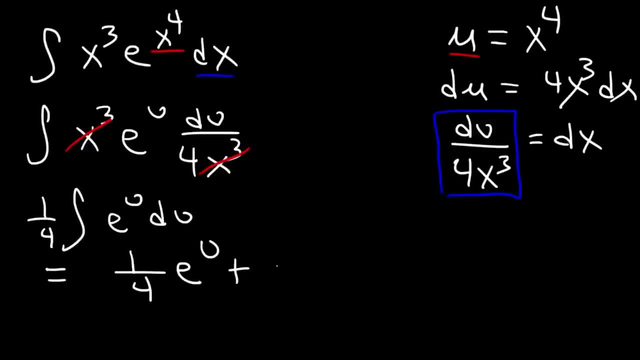 the antiderivative is 1 fourth e to the u plus c, And now let's replace u with x to the fourth. So this is the final answer: 1 fourth e raised to the x to the fourth plus c, And that's it. 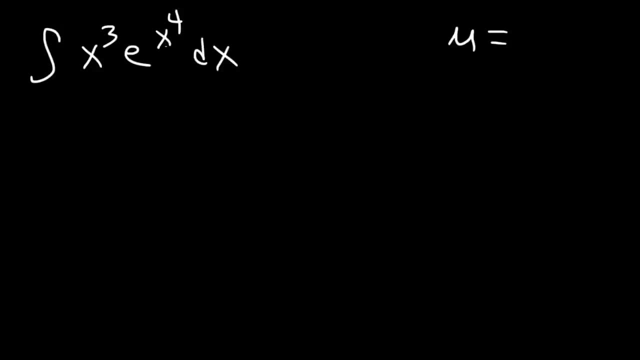 the fourth, du will be equal to 4x cubed, and that can get rid of the x cubed that we see here. So let's do that. Let's make u equal to x to the fourth. So du is going to be 4x cubed, dx, and then, as always, solve for. 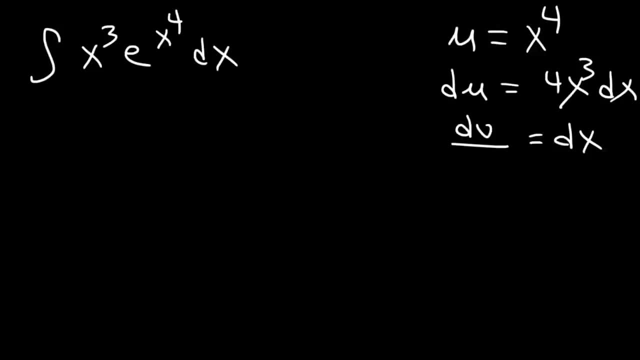 dx. If you don't do that, you can easily make a mistake. so I recommend, in this step, isolate dx. It'll save you a lot of trouble later on. So du is going to be- I mean dx is going to be- du over 4x cubed. Now let's replace x to the fourth with. 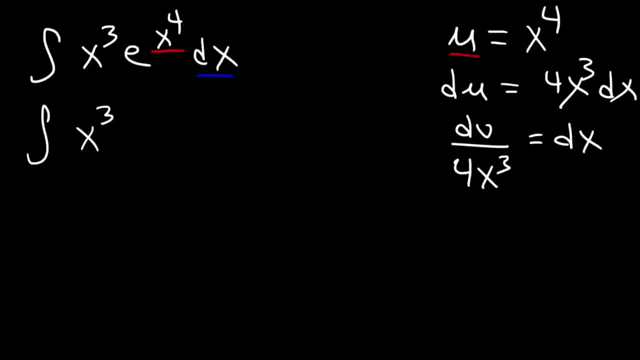 with u and let's replace dx with du over 4x cubed. So this is going to be e raised to the? u times: du over 4x cubed. So x cubed will cancel, which is good, and the 4 we can move it. 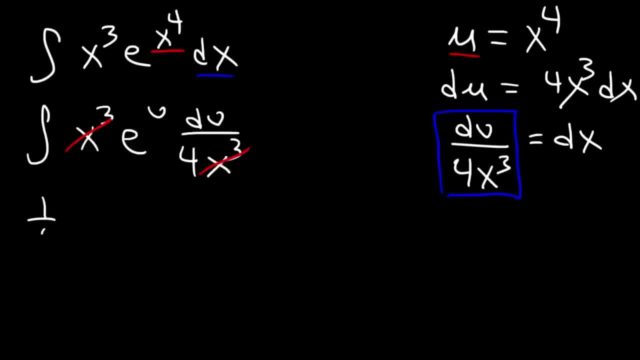 to the front Now, because it's in the bottom of the fraction, it's 1 over 4.. Now the antiderivative of e to the? u is simply e to the? u. So the final answer? well, not the final answer, but 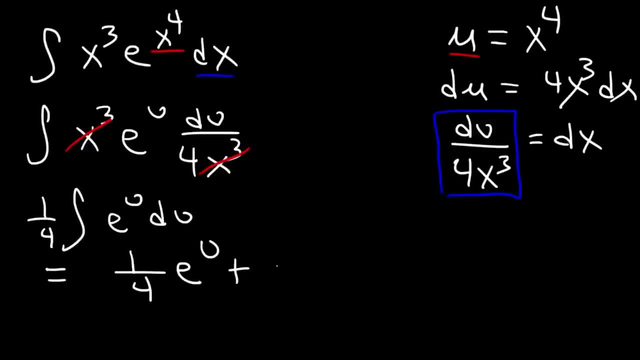 the antiderivative is 1 fourth e to the u plus c, And now let's replace u with x to the fourth. So this is the final answer: 1 fourth e raised to the x to the fourth plus c, And that's it. 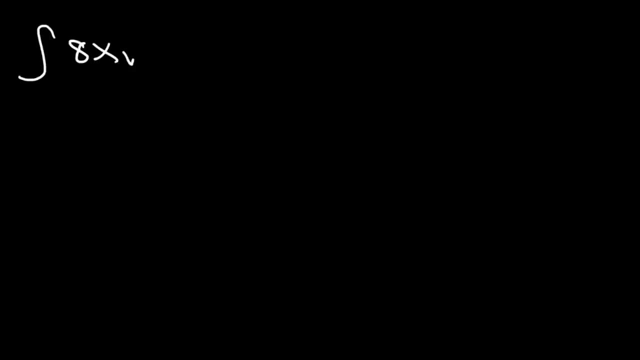 Here's another one. Find the indefinite integral of 8x times the square root of 40, minus 2x squared dx. So typically you want to make u equal to the stuff that's more complicated and that is the stuff on the inside of the square root. If we make u equal, 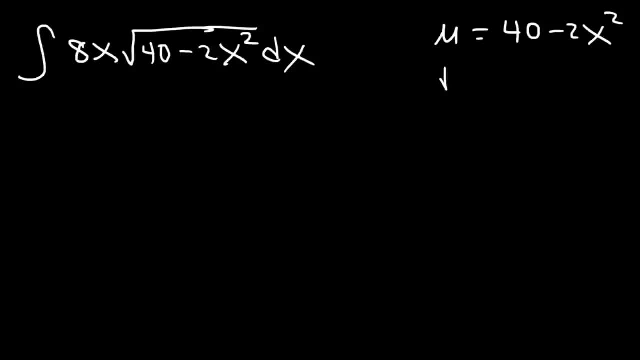 to 40 minus 2x squared, du is going to be: the derivative of 40 is 0, so we can ignore that, and the derivative of negative 2x squared that's going to be negative 4x dx. So isolating dx, we need to divide both sides by negative 4x, so it's du over negative 4x. 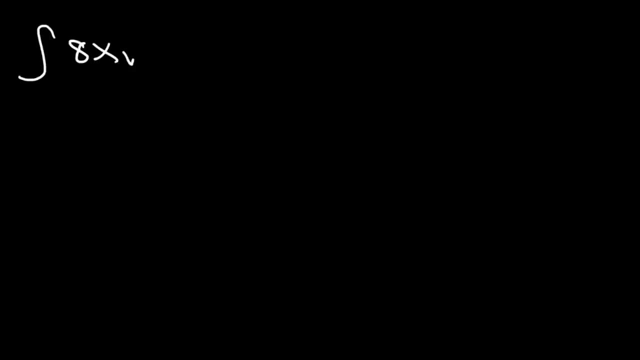 Here's another one. Find the indefinite integral of 8x times the square root of 40, minus 2x squared dx. So typically you want to make u equal to the stuff that's more complicated and that is the stuff on the inside of the square root. If we make u equal, 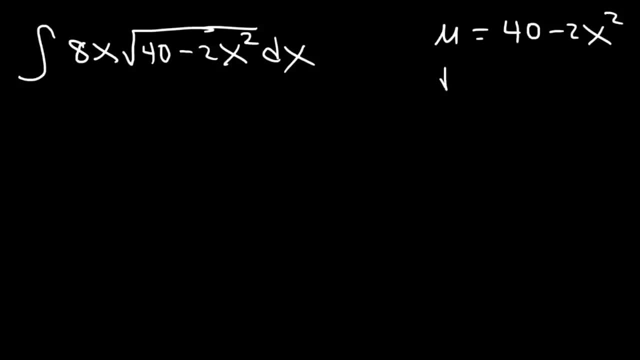 to 40 minus 2x squared, du is going to be: the derivative of 40 is 0, so we can ignore that, and the derivative of negative 2x squared that's going to be negative 4x dx. So isolating dx, we need to divide both sides by negative 4x, so it's du over negative 4x. 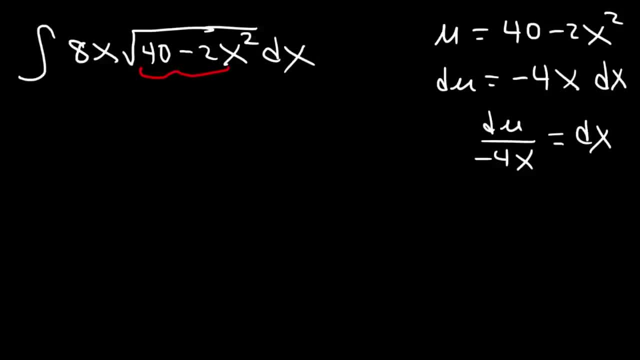 So let's replace this with u and this part, dx, with du over negative 4x, So it's going to be 8x times the square root of u times du divided by negative 4x. 8x divided by negative 4x times u. 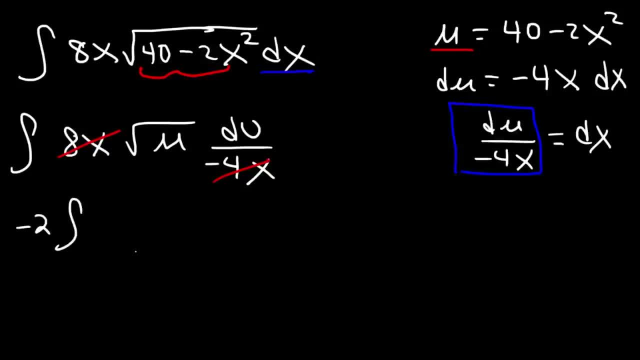 4x is negative 2.. And I'm going to write that in front. The square root of u is the same as u to the 1 half. So now we can use the power rule: 1 half plus 1 is 3 over 2.. And then we could divide. 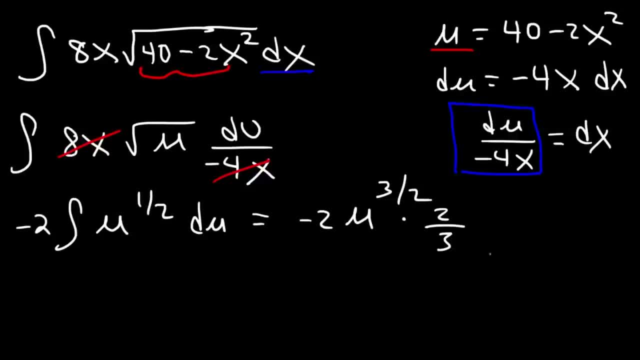 by 3 over 2 or multiply by 2 over 3, which is the better option? So negative 2 times 2 thirds, that's negative 4 over 3.. Now the last thing we need to do is replace the u variable with 40. 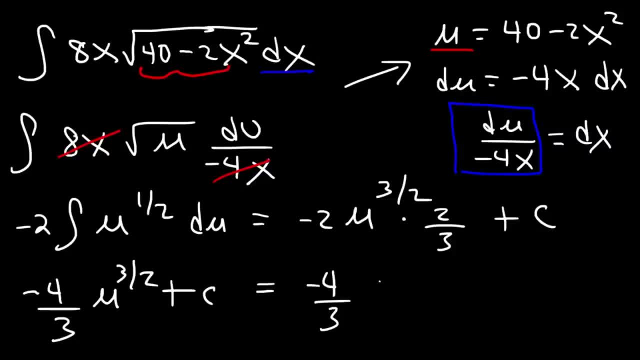 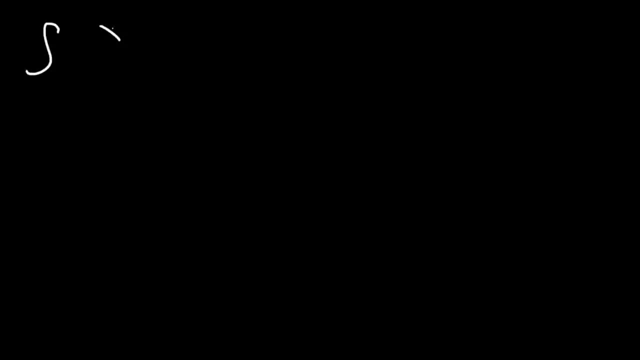 minus 2x squared. So the final answer is negative: 4 over 3, 40 minus 2x squared raised to the 3 over 2 plus c, And that's all we need to do. Let's work on some more problems. Feel free to pause. 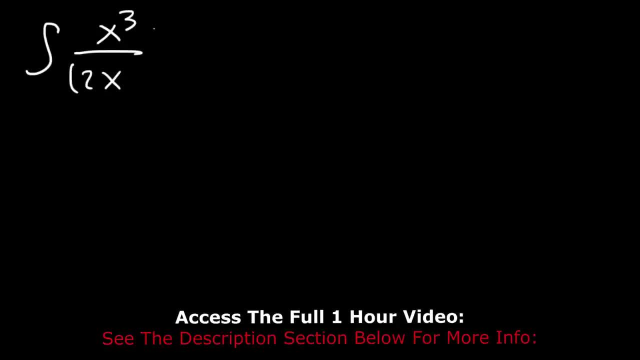 the video and try this one. Integrate x cubed divided by 2 plus x to the 4th, raised to the 2nd power. Now, typically it's better to make u equal to the stuff that has the higher exponent. 4 is higher than 3.. So let's make u equal. 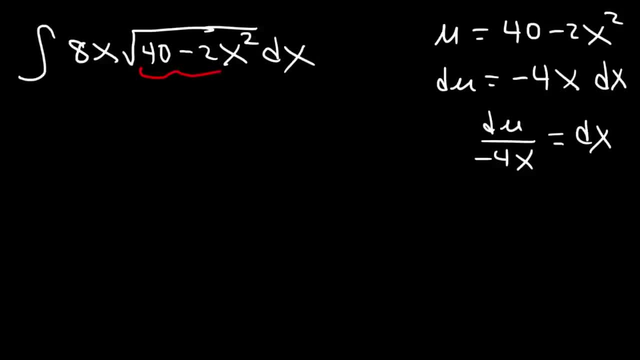 So let's replace this with u and this part dx, with du over negative 4x. So it's going to be 8x times the square root of u times du divided by negative 4x. 8x divided by negative 4x is going to be: 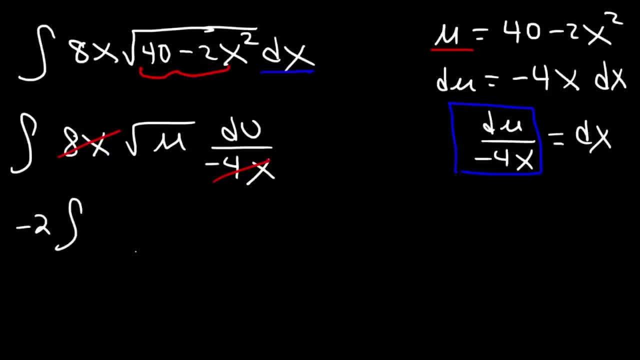 negative 2.. And I'm going to write that in front: The square root of u is the same as u to the 1 half. So now we can use the power rule: 1 half plus 1 is 3 over 2, and then we could divide by 3 over 2, or 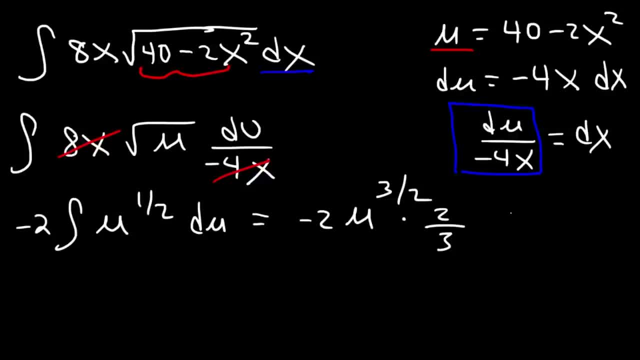 multiply by 2 over 3, which is the better option. So negative 2 times 2 thirds, that's negative 4 over 3.. Now the last thing you need to do is to find the integral of x squared, So you're going to need to divide this by 2 over 3, so it's going to be 2 over 4x plus 2 over 3.. 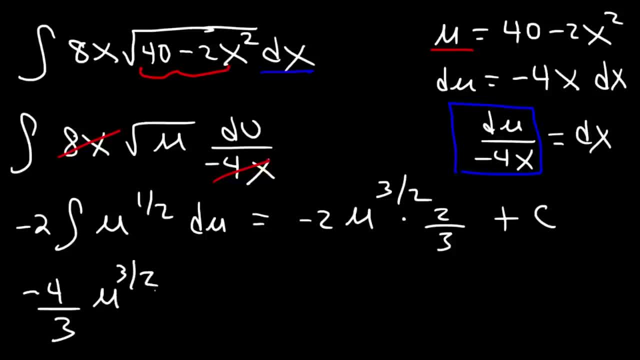 So negative 2 times 2 thirds, that's negative 4 over 3.. Now the last thing you need to do is to calculate the integral of x squared. dx is replace the u variable with 40 minus 2x squared. So the final answer is negative 4 over 3,. 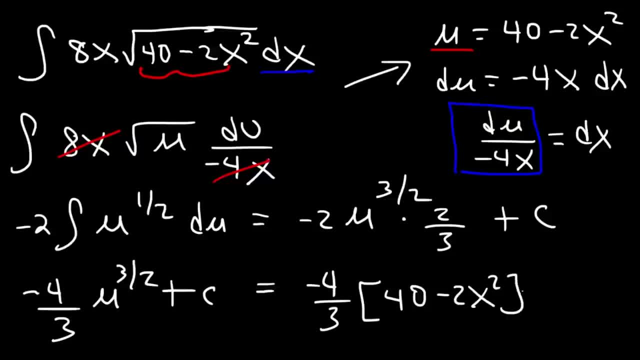 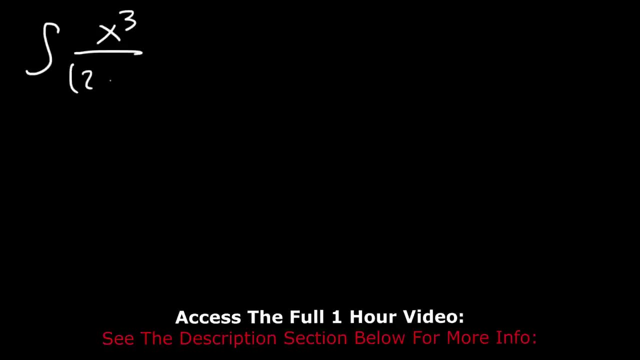 40 minus 2x, squared raised to the 3 over 2 plus c. And that's all we need to do. Let's work on some more problems. Feel free to pause the video and try this one. So integrate x cubed divided by 2 plus x to the 4th, raised to the 2nd power. 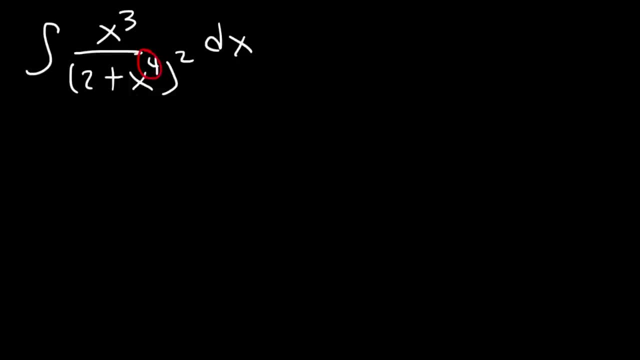 Now, typically it's better to make u equal to the stuff that has the higher exponent. 4 is higher than 3.. So let's make u equal to 2 plus x to the 4th. du is going to be the derivative of x to the 4th. 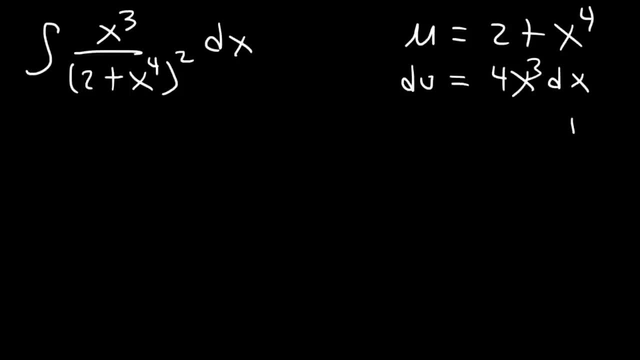 so that's 4x squared. du is going to be the derivative of x to the 3rd power times dx And as always, I recommend that you solve for dx, just to avoid mistakes. So let's replace 2 plus x to the 4th with u. 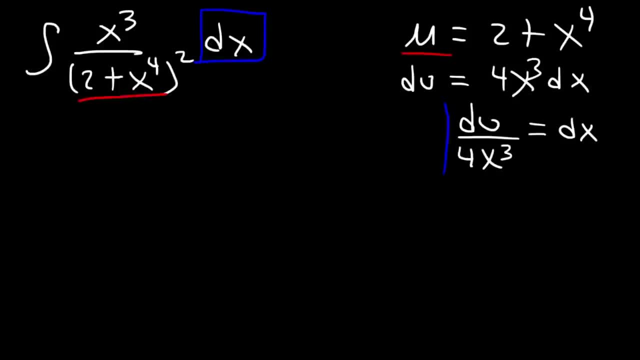 and let's replace dx with this thing that we have here. So we're going to have x to the 3rd on top, u squared on the bottom and dx is du over 4x cubed. And if you don't know how to do this, 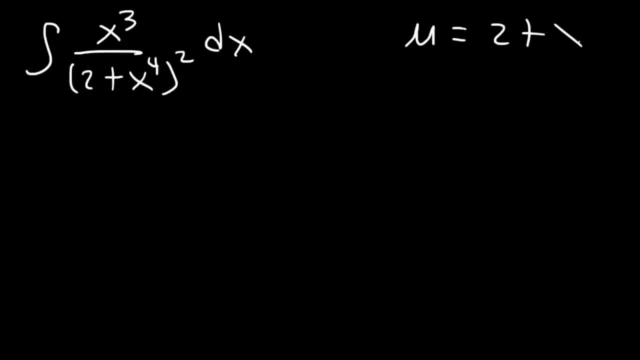 to 2 plus x to the 4th, du is going to be the derivative of x to the 4th, So that's 4x squared to the 3rd power times dx. And as always, I recommend that you solve for dx, just to avoid. 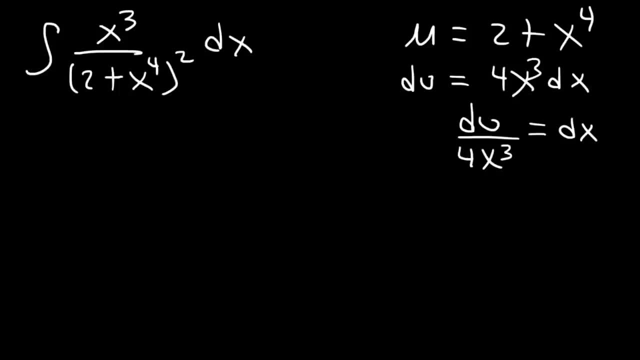 mistakes. So let's replace 2 plus x to the 4th with u And let's replace dx with this thing that we have here. So we're going to have x to the 3rd on top, u squared on the bottom and dx is du over. 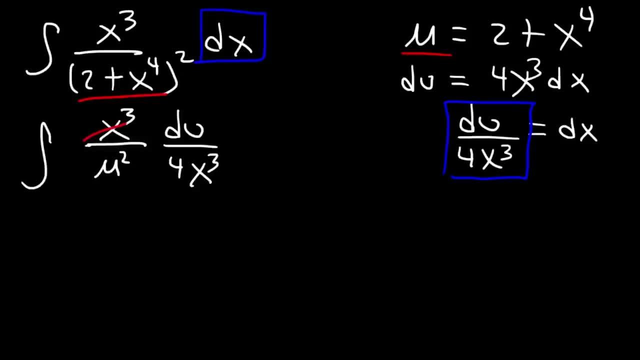 4x cubed. If you do it this way, as you can see, the remaining x variables will cancel out nicely. So this 4 is on the bottom, Let's move it to the front. So it becomes 1, 4th anti-derivative. 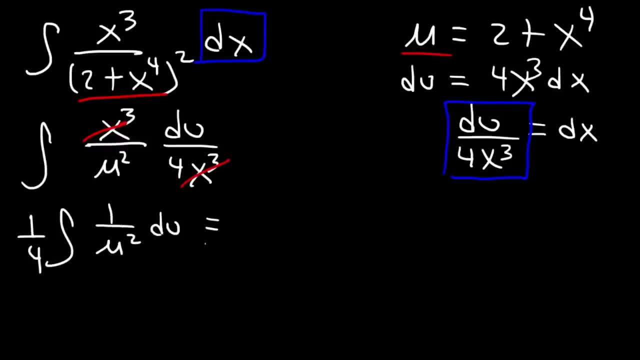 1 over u squared du, And so let's move the u squared from the bottom to the top. So this is going to be 1 4th integration of u to the negative 2 du, And now we can use the power rule. 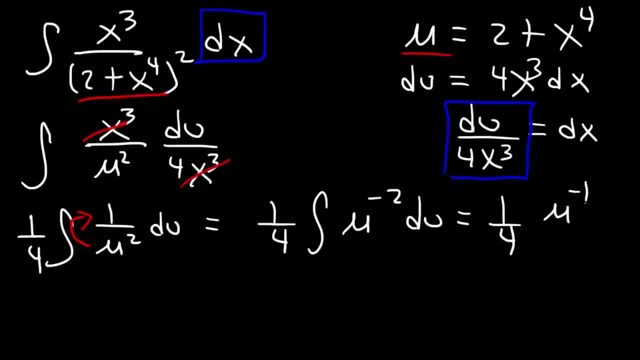 So if we add 1 to negative 2, that's going to be 1. 4th, So that's going to be 1 over u squared, And then we need to divide by negative 1.. So now let's bring this variable back to the bottom to make the negative exponent positive. 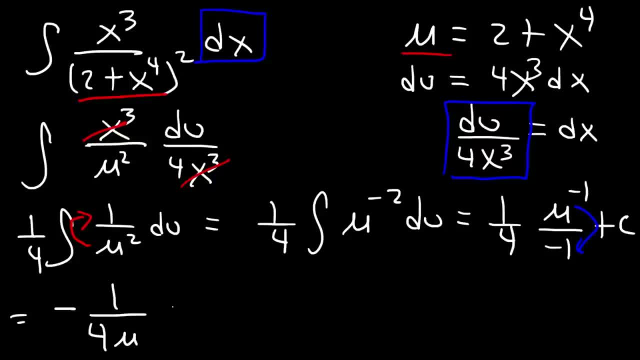 So it's negative, 1 over 4u plus c. Now let's replace u with what we said it equal to in the beginning. So I'm going to need a bigger fraction. So u is 2 plus x, squared. Okay, x to the fourth and then plus c. So this is the final answer. Let's integrate sine to: 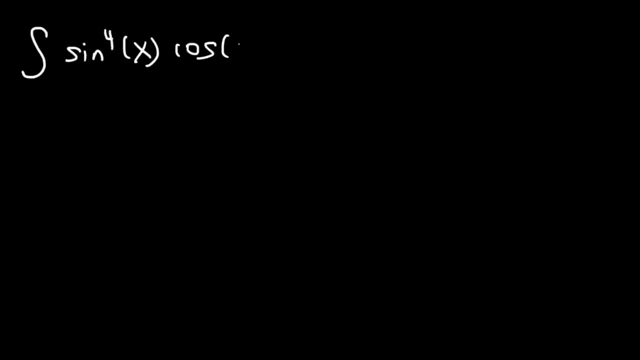 the fourth of x times cosine of x dx. So go ahead and find the antiderivative of this trigonometric function. So if we make u equal to cosine, du will be negative sine dx. That will only cancel one of the sine variables And it's best to make u. 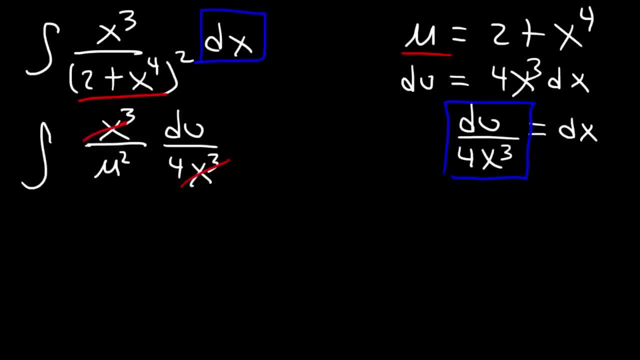 you can do it by looking at this. As you can see, the remaining x variables will cancel out nicely. So this 4 is in the bottom. Let's move it to the front. so it becomes 1. 4th anti-derivative: 1 over u squared du. 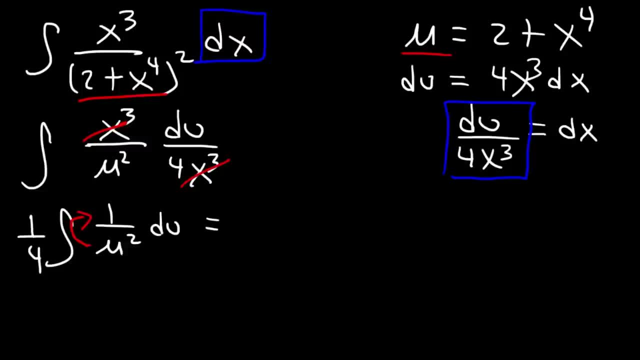 And so let's move the u squared from the bottom to the top. So this is going to be 1. 4th integration of u to the negative 2 du, And now we can use the power rule. So if we add 1 to negative 2,. 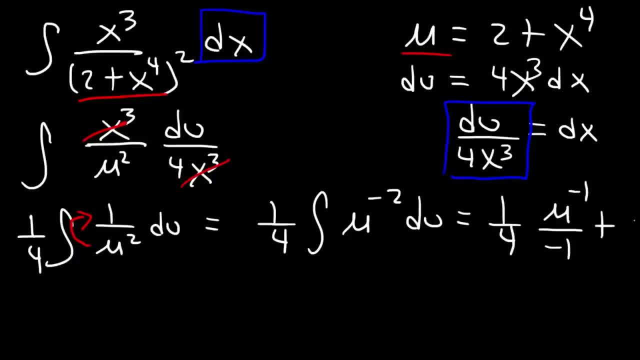 that's going to be negative 2.. So that's going to be negative 2.. So that's going to be negative 2.. And then we need to divide by negative 1.. So now let's bring this variable back to the bottom. 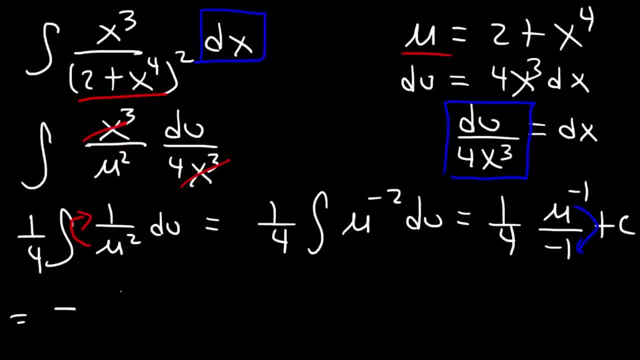 to make the negative exponent positive, So it's negative 1 over 4u plus c. Now let's replace u with what we said. it equal to in the beginning, So I'm going to need a bigger fraction. So u is 2 plus x to the 4th. 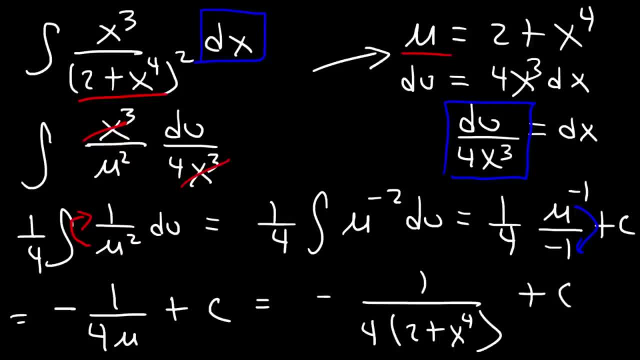 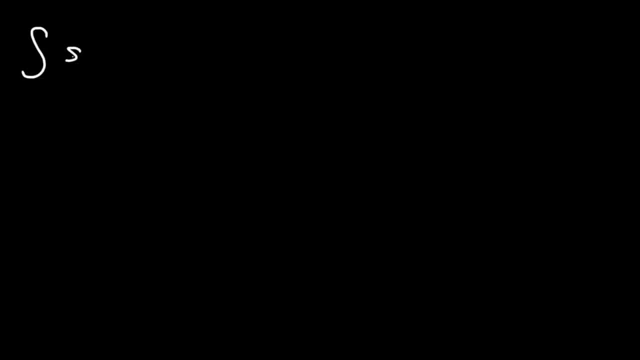 and then plus 2.. Let's see. So this is the final answer. Let's integrate sine to the 4th of x times cosine of x dx. So go ahead and find the anti-derivative of this trigonometric function. 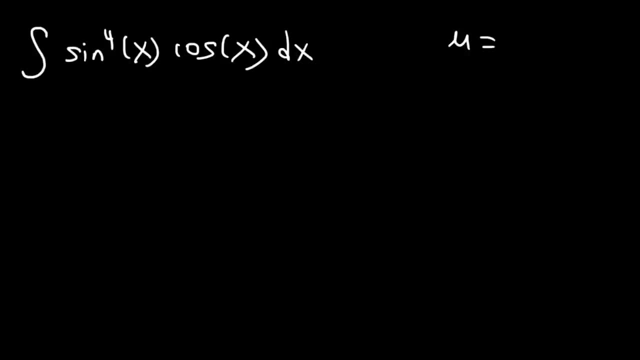 So if we make u equal to cosine, du will be negative sine dx, That will only cancel 1, and then we'll have the exponent of the sine variables, And it's best to make u equal to the trig function that you have more of. 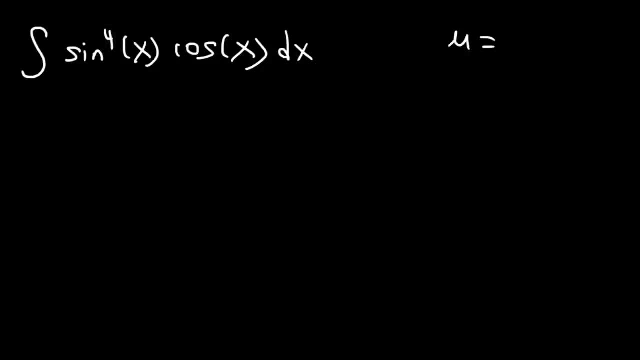 We have 4 sines and only 1 cosine, So it's best to make u equal to sine x And du will be equal to cosine x, And since there's only 1 cosine, this will be completely canceled. Solving for dx is going to be du divided by cosine x. 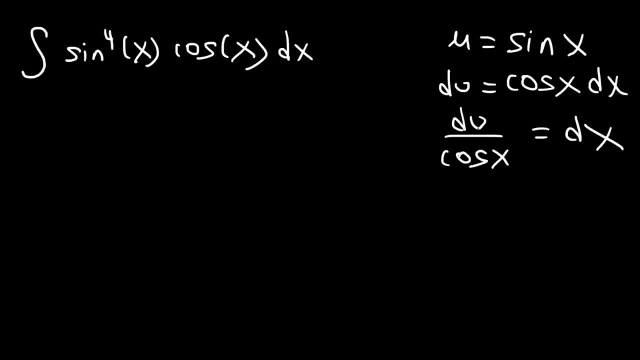 And don't forget that last step: Always isolate dx, Always isolate dx. So let's replace this with u. So this is going to be u to the 4th times. cosine x and dx is du divided by cosine. So we could cancel cosine x. 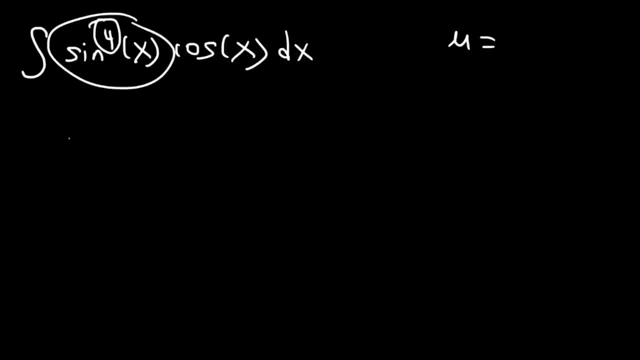 equal to the trig function that you have more of. We have four sines and only one cosine, So it's best to make u equal to sine x And du will be equal to cosine x, And since there's only one cosine, this will be completely cancelled. Solving for: 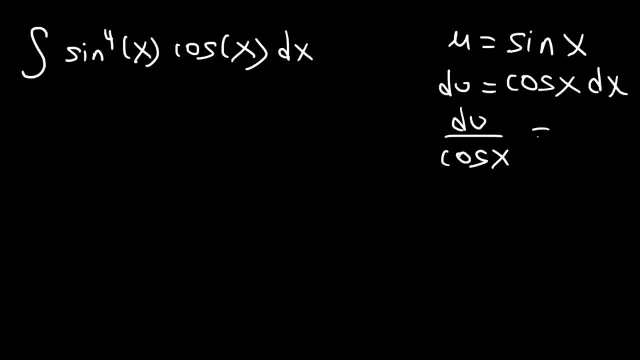 dx is going to be du divided by cosine x. And don't forget that last step: Always isolate the cosine. So let's replace this with u. So this is going to be u to the fourth times: cosine x and dx is du divided by cosine. So we could cancel cosine x And so we're left with the. 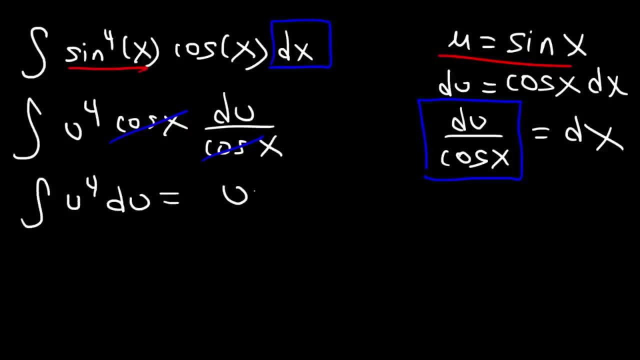 indefinite integral of u to the fourth du, Using the power rule, 4 plus 1 is 5 and then divide by 5.. So we have one-fifth u to the 5 plus c, And the last thing we need to do is: 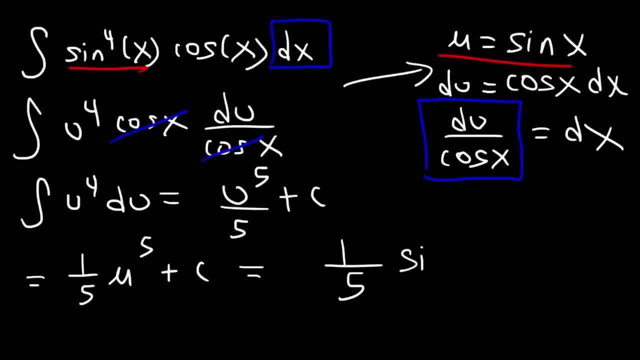 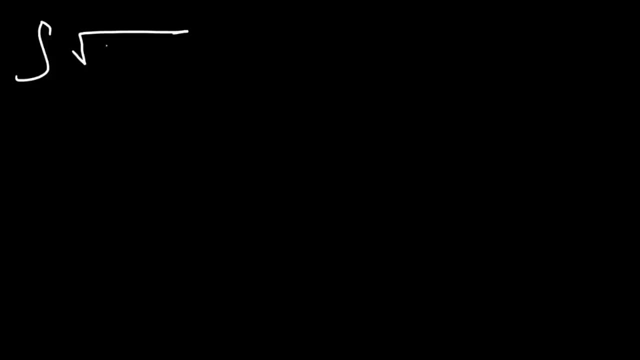 replace u with sine x, So it's one-fifth sine raised to the fifth power of x plus c. And that concludes this problem. Now, what would you do if you have to integrate the square root of 5x to the 5th? 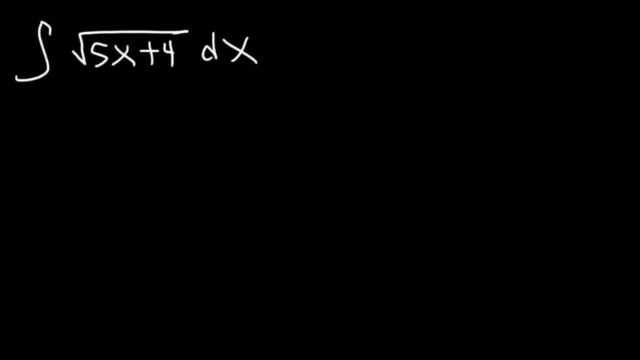 Now, in this problem, all we could do is set u equal to 5x plus 4.. There's nothing else that we can do, So let's go ahead and do this. The derivative of 5x is going to be 5 and then times dx, So isolating dx, it's going to be du over 5.. 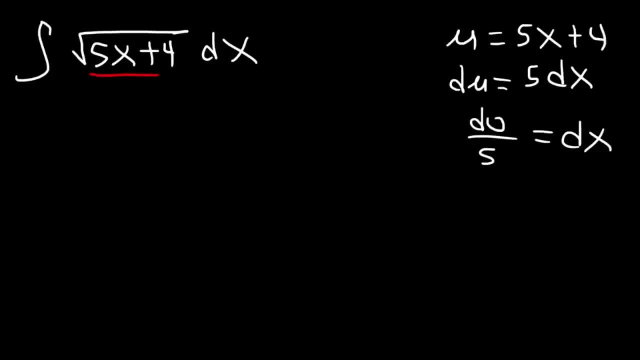 So, just like before, we're going to replace 5x plus 4 with u and dx with du over 5.. So then this becomes the square root of u and dx is du divided by 5. And move the 5 to the front. So this is one-fifth, and then, instead of the square root of u, 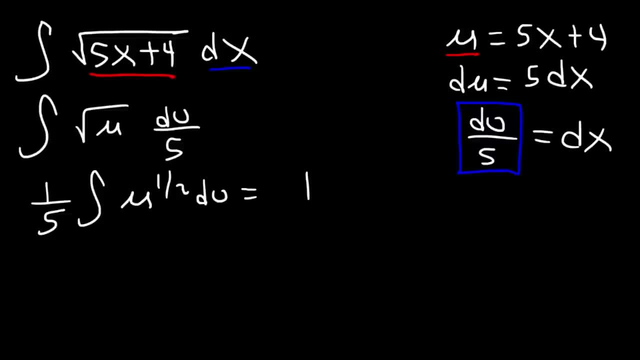 we're going to write it as u to the one-half. So now let's use the power rule: One-half plus 1, that's going to be 3 over 2.. And if you divide it by 3 over 2,, 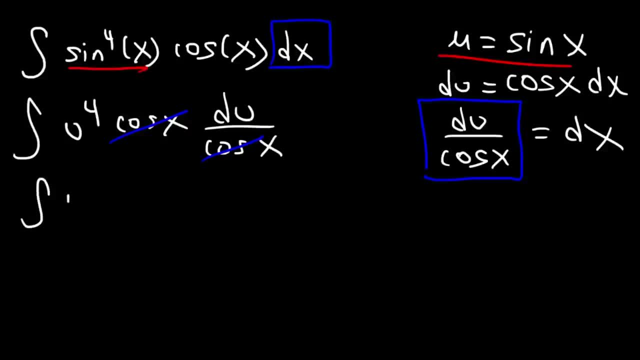 And so we're left with the indefinite integral of u to the 4th du. Using the power rule, 4 plus 1 is 5. And then divide by 5., And that's it. so we have one-fifth u to the 5 plus c, and the last thing we need to do is: 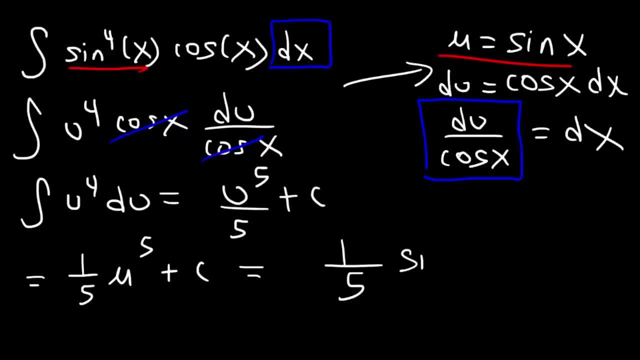 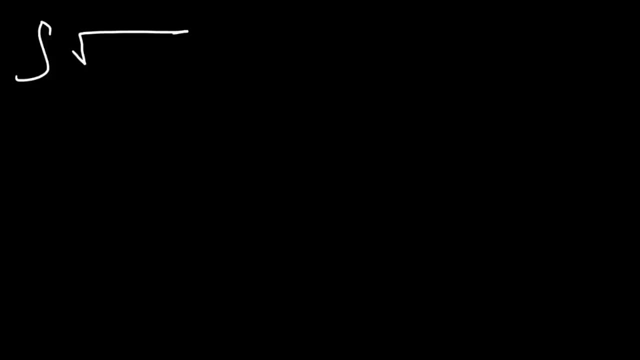 replace u with sine x, so it's one-fifth sine raised to the fifth power of x plus c. and that concludes this problem. now, what would you do if you have to integrate the square root of 5x plus 4 now in this problem? all we could do is set u equal to 5x plus 4. there's nothing. 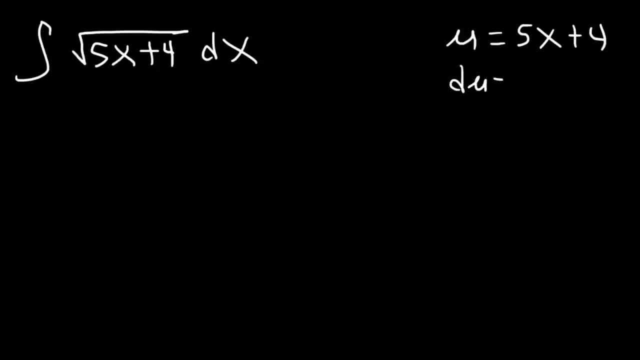 else that we can do, so let's go ahead and do this. the derivative of 5x is going to be 5 and then times dx, so isolating dx, it's going to be du over 5. so, just like before, we're going to replace 5x plus 4 with u and dx with du. 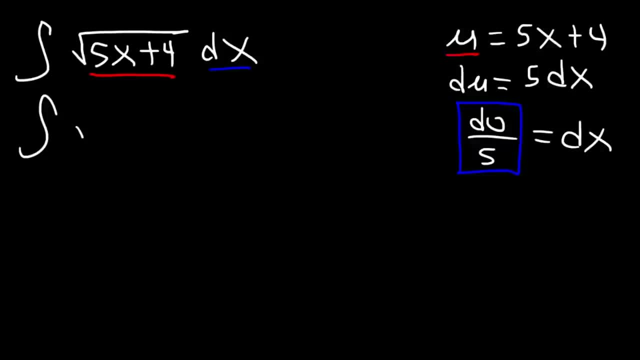 over 5. so then this becomes the square root of u and dx is du divided by 5, and move the 5 to the front, so this is one-fifth, and then instead of the square root of u, we're going to write as u to the one-half. so now let's use the power rule one-half. 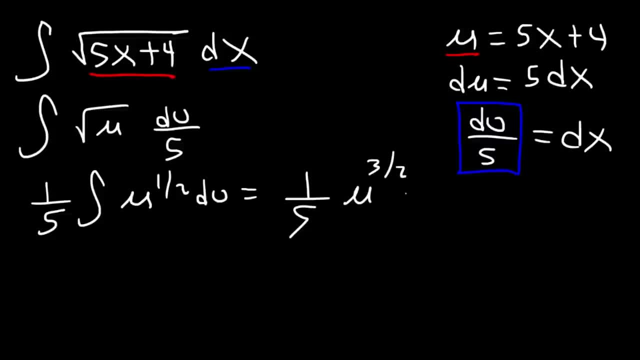 plus 1, that's going to be 3 over 2, and if you divide it by 3 over 2, what I would recommend is multiply the top and the bottom by two-thirds. so the threes in the bottom will cancel and the twos will cancel as well. so in 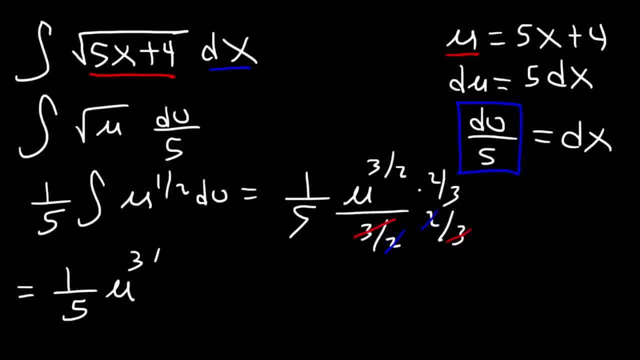 the end, you get one-fifth? u to the three-halves, times 2 over 3, which becomes 2 over 15? u to the three-half. and let's not forget the constant of integration plus c. so now to write the final answer. all we need to do is: 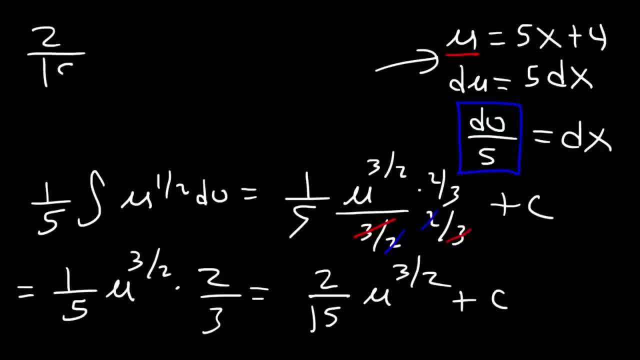 replace u with 5x plus 4, so it's 2 over 15, 5x plus 4 raised to the three over 2 plus c, and so that's the solution. so, as you can see, u substitution is not very difficult once you get the hang of it. as. 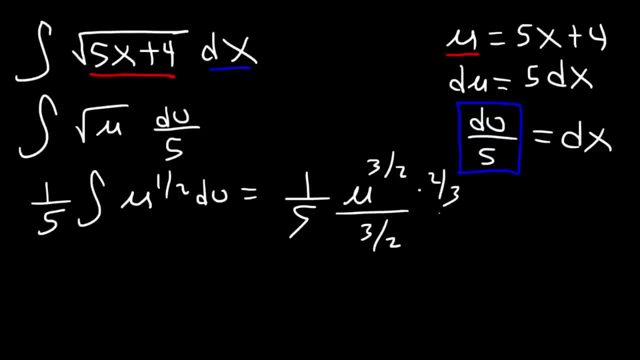 what I would recommend is: multiply the top and the bottom by two-thirds, So the threes in the bottom will cancel and the twos will cancel as well. So in the end you get one-fifth? u to the three-halves times 2 over 3, which becomes 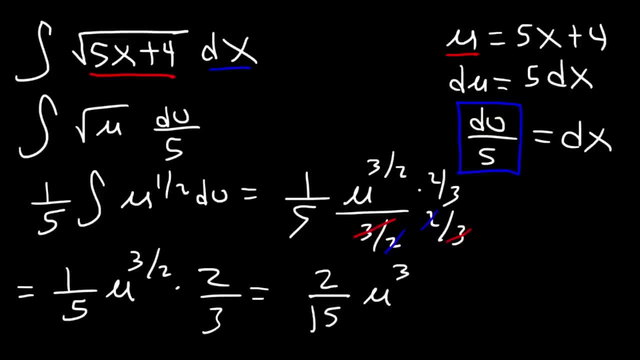 2 over 15, u to the three-half, And let's not forget the constant of integration plus c. So now to write the final answer. all we need to do is replace u with 5x plus 4.. So it's 2 over 15.. 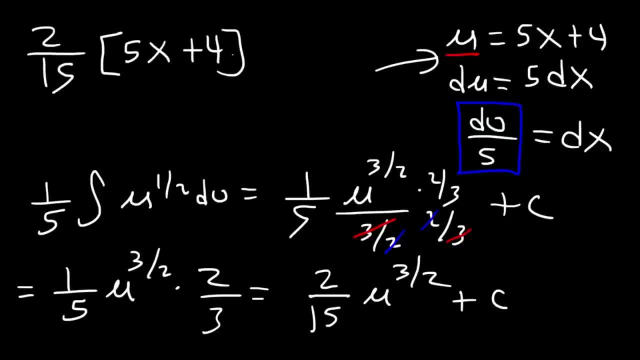 5x plus 4 raised to the 3 over 2 plus c, And so that's the solution. So, as you can see, u substitution is not very difficult once you get the hang of it, As long as you do a few problems and get used to. 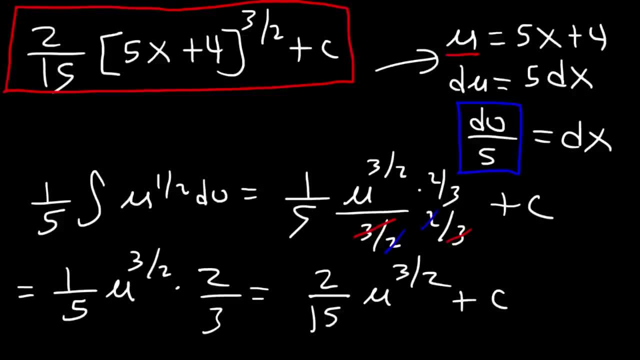 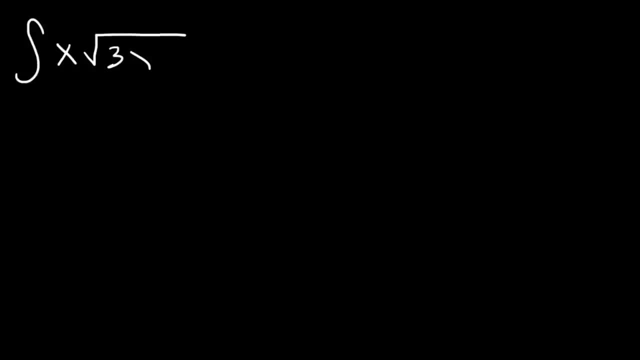 the method and the techniques employed here, it's a piece of cake. Now, this problem is a little bit different from the others. Go ahead and try it. I recommend that you pause the video and give this one a go. So let's set u equal to the stuff that's more complicated: 3x plus 2.. Now du. 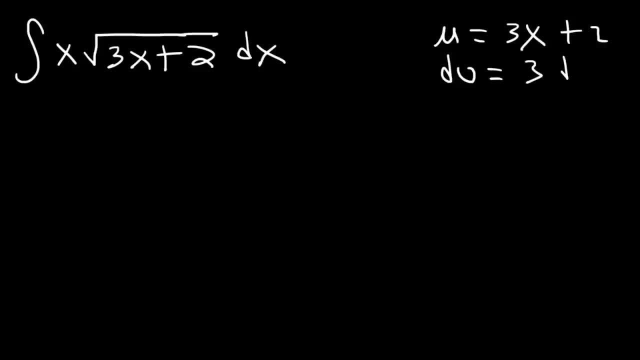 that's going to be the derivative of 3x, which is 3 times dx, So isolate in dx it's going to be du over 3.. And this time this x variable will not cancel. So notice that the x variables are of the same degree And when you see this situation it indicates that 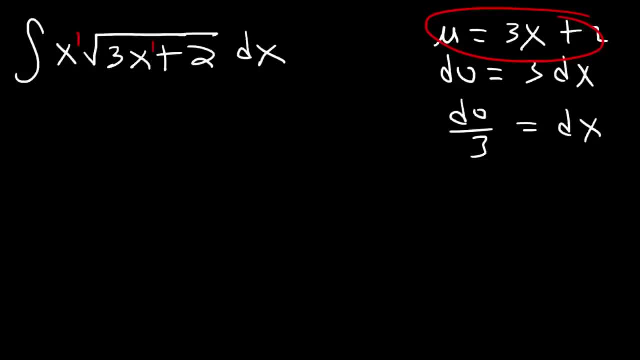 in this expression. you need to solve for x, So isolating x. I need to move the 2 to the other side. So I have: u minus 2 is equal to 3x And then divided by 3, u minus 2 over 3 is x. 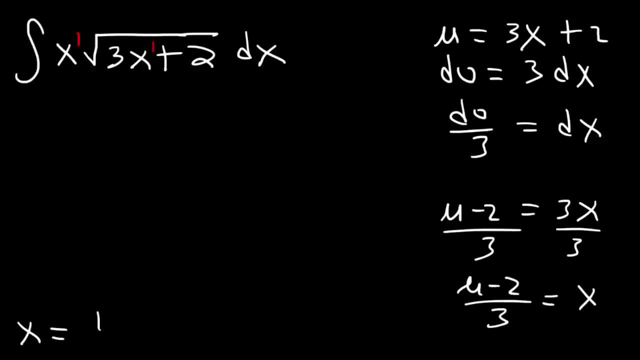 which you can write it. as you can say: x is one-third u minus 2, which I think looks a lot better. Now, keep in mind: in order to perform u substitution, we need to eliminate every x variable in this expression. If we replace 3x plus 2 with u and then dx with du over 3,. 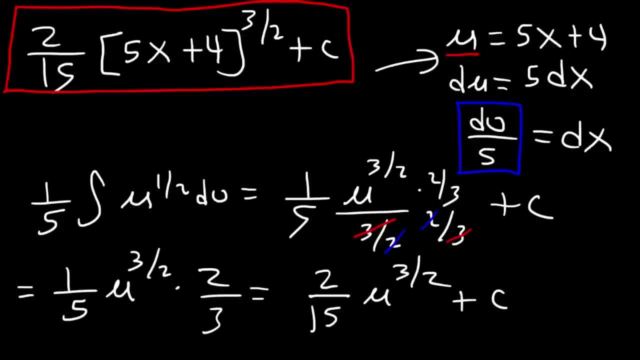 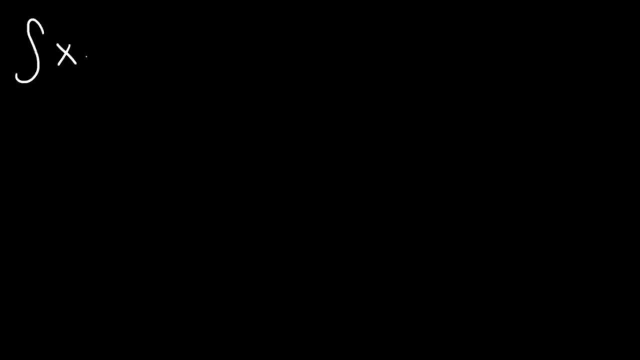 long as you do a few problems and get used to the method and the techniques employed here, it's a piece of cake. now this problem is a little bit different from the others. go ahead and try it. I recommend that you pause the video and give this one ago. so let's set. 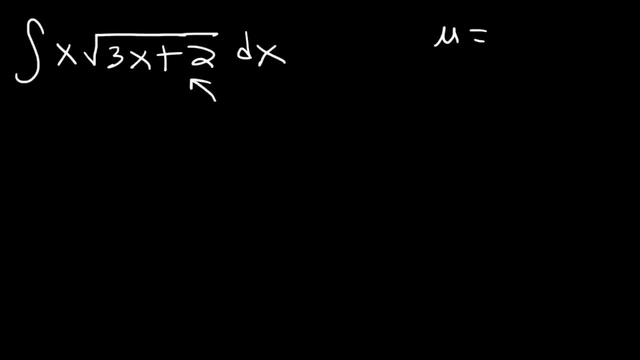 u equal to the stuff that's more complicated: 3x plus 2, now du, that's going to be the derivative of 3x, which is 3 times dx, so isolate in dx it's going to be du over 3, and this time this x variable will not cancel, so notice. 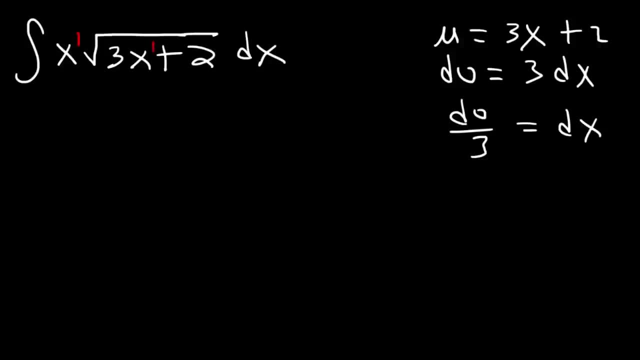 that the x variables are of the same degree. when you see the situation, it indicates that in this expression you need to solve for x, so isolating x. I need to move the two to the other side. so I have: u minus 2 is equal to 3x, and then 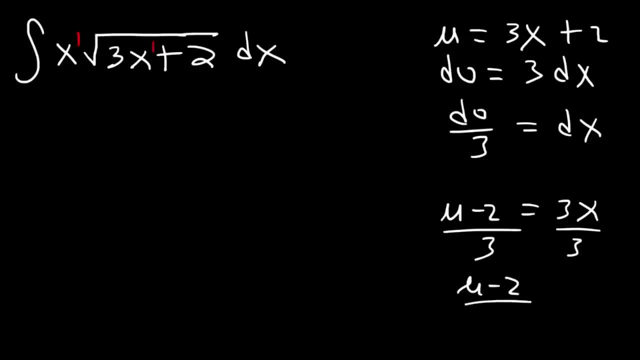 divided by 3, u minus 2 over 3 is x, which you can write it as you can say: x is 1. third, u minus 2, which i think it looks a lot better now. keep in mind: in order to perform use substitution needs to eliminate every X variable in this. 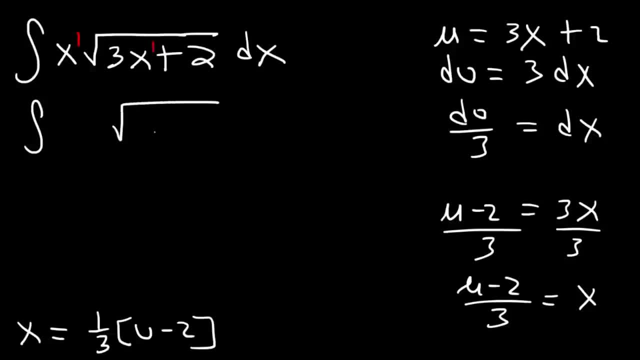 expression. if we replace 3x plus 2 with you and then DX with du over three, this X will still be here, and so that's why we need to solve for X and this expression. so make sure to do that if these two are of the same degree. so this is going to be one-third. i'm going to 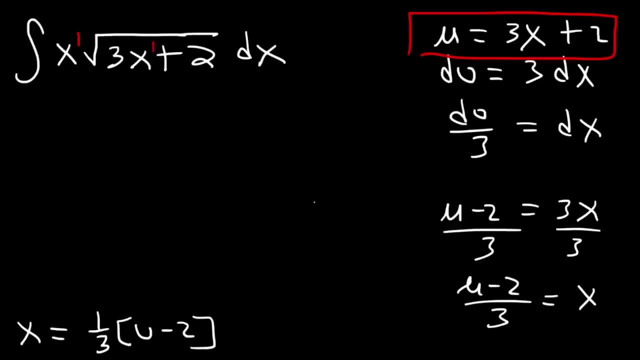 have to rewrite it because i can't fit it in here. so let's replace experts with one-third you minus two, and then we have the square root of you, and DX is du divided by 3. so one-third times du over 3, that's going to be du over 9. so I'm 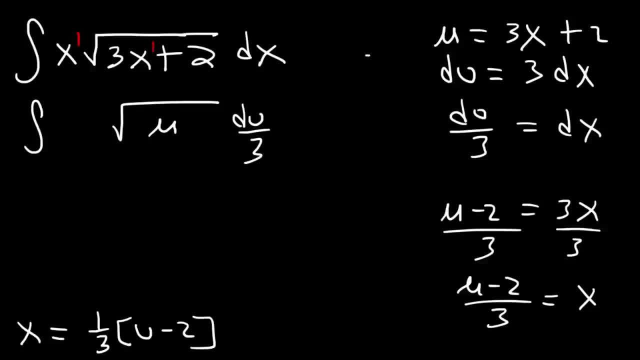 this x will still be here, And so that's why we need to solve for x in this expression. So make sure to do that if these two are of the same degree. So this is going to be one-third. I'm going to have to rewrite it because I can't fit it in here. 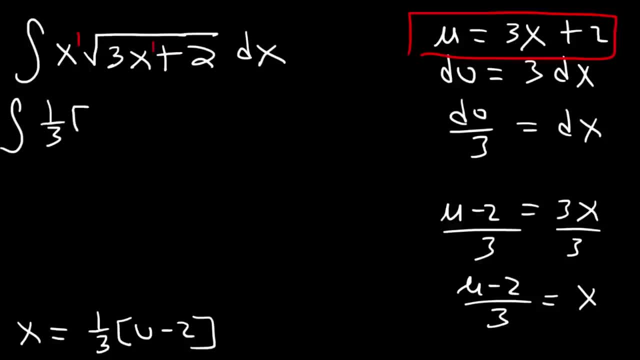 So let's replace x first with one-third u minus 2, and then we have the square root of u and dx is du divided by 3.. So, So 1, 3rd times du over 3, that's going to be du over 9.. 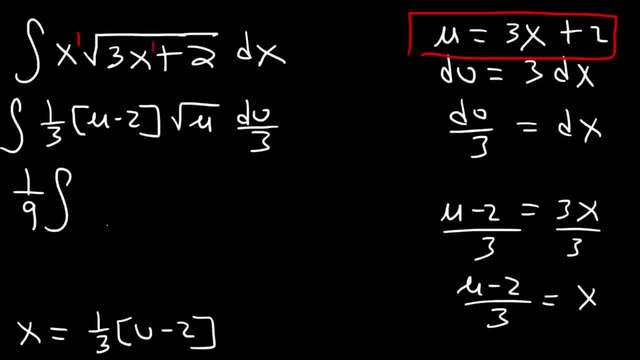 So I'm going to take the 1? 9th and move it to the front, And then I have u minus 2, and the square root of u is u to the 1 half and then du. So now we only have the u variable. 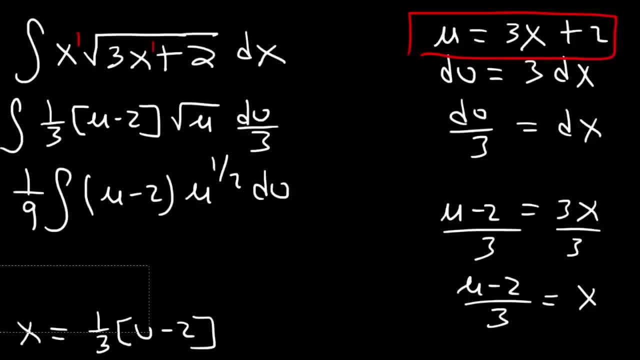 In this form we can integrate it. Now. the next thing we need to do is distribute u to the 1 half, to u minus 2.. So u to the 1st power times, u to the 1 half. we need to add 1 and 1 half. 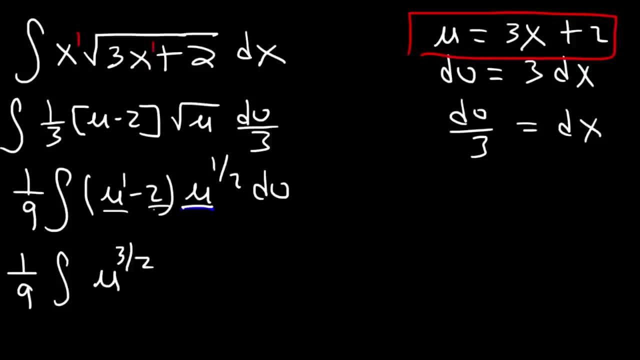 That's going to be u to the 3 over 2.. And then if we multiply negative 2 by u to the 1 half, that's negative 2, u to the 1 half, And then times du. So now we can find the antiderivative of each one. 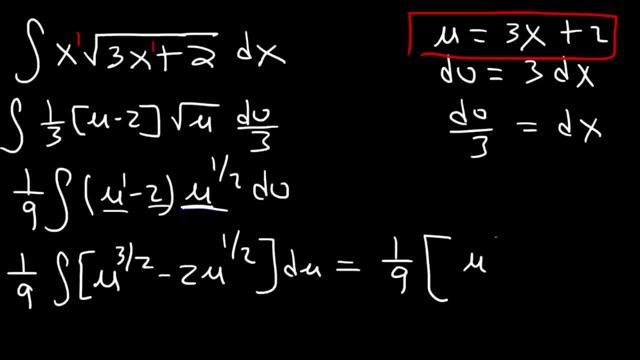 So for u to the 3 halves, it's going to be 3 over 2 plus 1, which is 5 over 2.. And instead of dividing it by 5 over 2, we're going to multiply it by 2 over 5.. 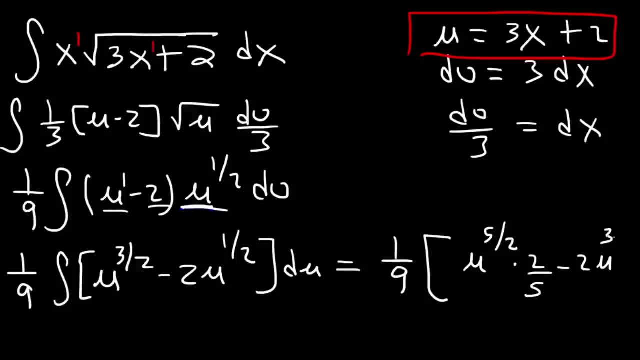 And for u to the 1, half. 1 half plus 1 is 3 over 2, and then we're going to multiply it by 2- 3rds, And then we need to add plus c. So now let's distribute 1 over 9 to everything on the inside. 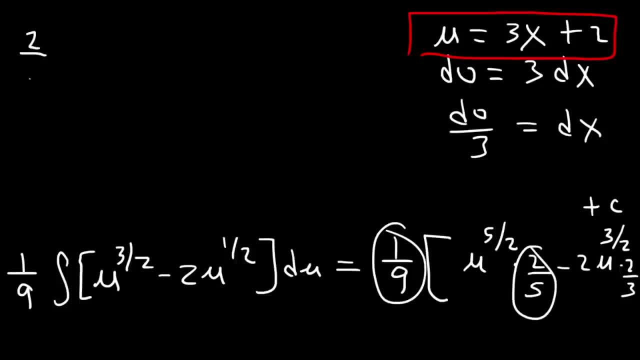 So 1 over 9 times 2 over 5. That's going to be 2 over 45 times u raised to the 5 over 2.. And then we have 1 ninth times. this is basically negative 4. 3rds. 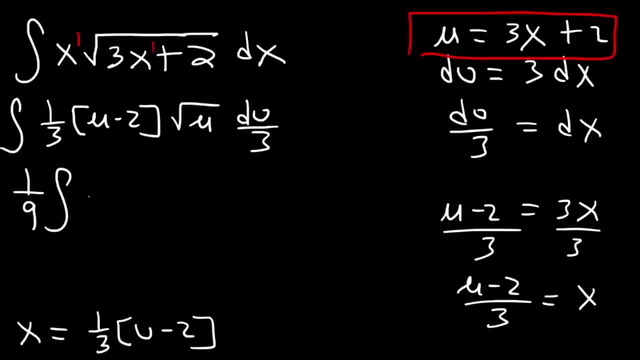 going to take the one-ninth and move it to the front, and then I have you minus two and the square root of you is you to the one-half, and then do you. so. now we only have the u variable. in this form we can integrate it. 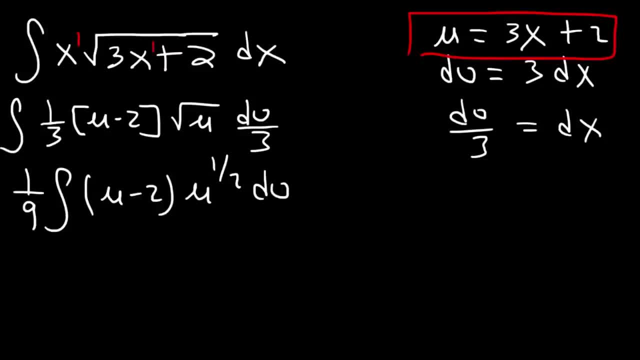 now the next thing we need to do is distribute you to the one-half, to you minus two. so you to the first power times, you to the one-half. we need to add one and one-half. that's going to be you to the three over two, and then, if we 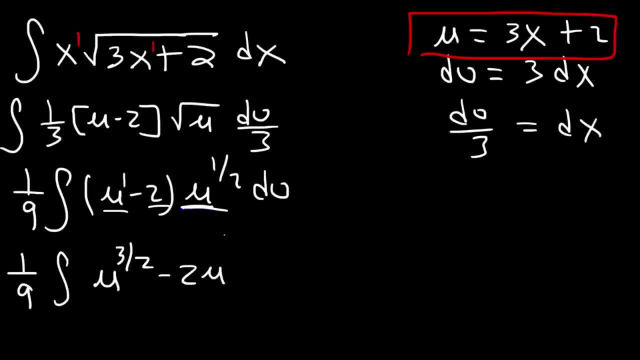 multiply negative 2 by you to the one-half, that's negative 2, you to the one-half and then times du. so now we can find the antiderivative of each one. so for you to the three halves is going to be 3 over 2 plus 1, which is 5 over 2, and 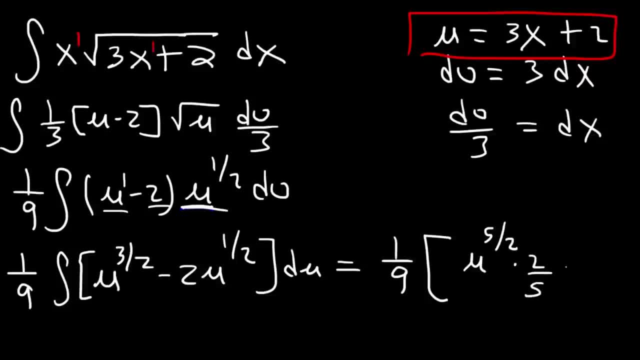 instead of dividing it by 5 over 2, we're going to multiply by 2 over 5, and for you to the one-half, 1, half plus 1 is 3 over 2, and then we're going to multiply by two-thirds and then we need to add plus C. so now let's distribute 1 over 9 to: 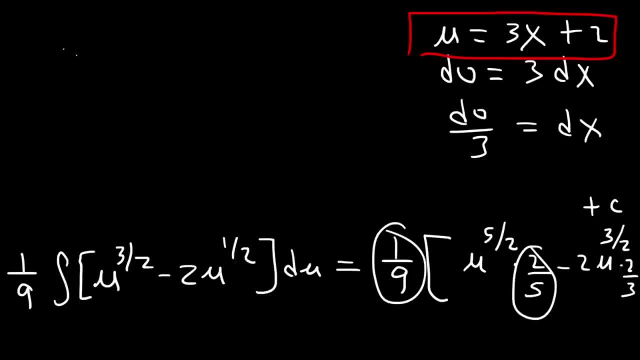 everything on the inside. so 1 over 9 times 2 over 5, that's going to be 2 over 45 times u. raised to the 5 over 2, and then we have one knife times. this is basically negative 4 thirds. so that's going to be negative 4. 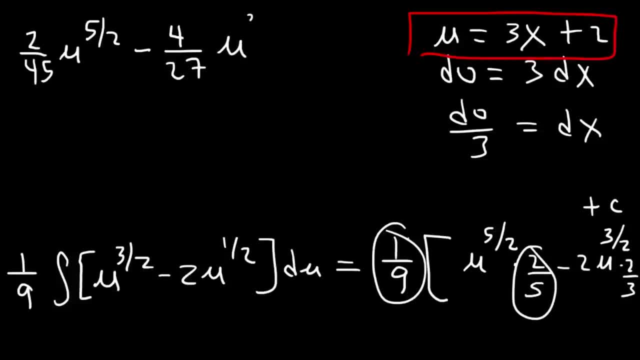 over 27, and that's u to the 3 over 2, and then plus C. so now let's replace u with 3x plus 2, so the final answer is going to be 2 over 45, 3x plus 2 raised to the. 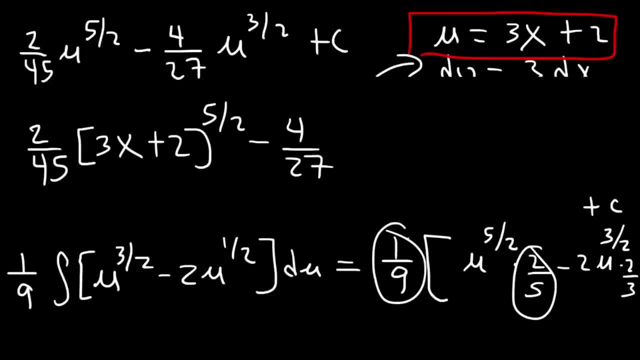 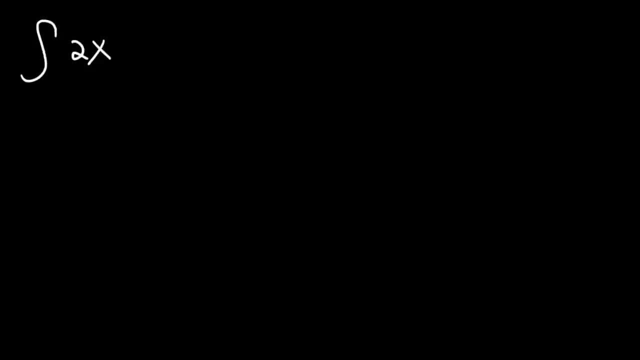 5 over 2 minus 4 over 27 times 3x plus 2 raised to the 3 over 2 plus C, and that is it. now let's work on. this example is very similar to the last one, so you can try if you want more practice. 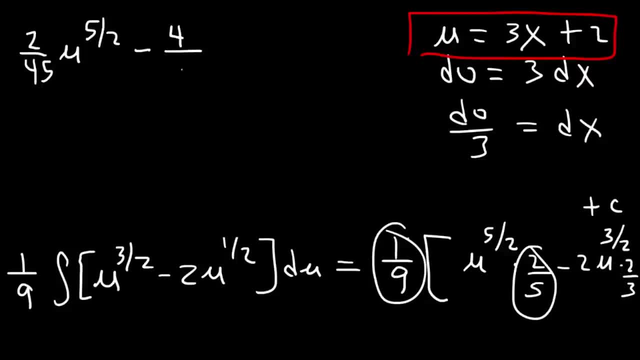 So that's going to be negative 4 over 27.. And that's u to the 3 over 2, and then plus c. So now let's replace u 3x plus 2.. So the final answer is going to be 2 over 45,, 3x plus 2 raised to the 5 over 2, minus 4 over 27 times 3x plus 2 raised to the 3 over 2, plus c. 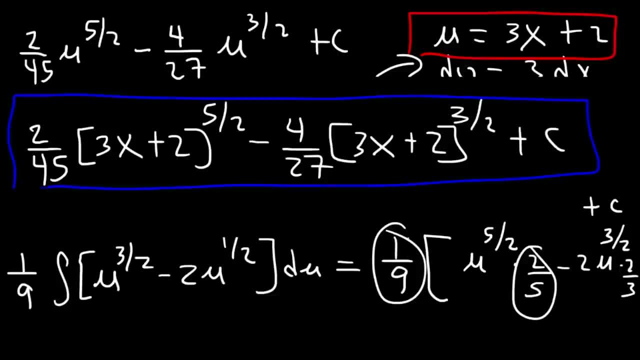 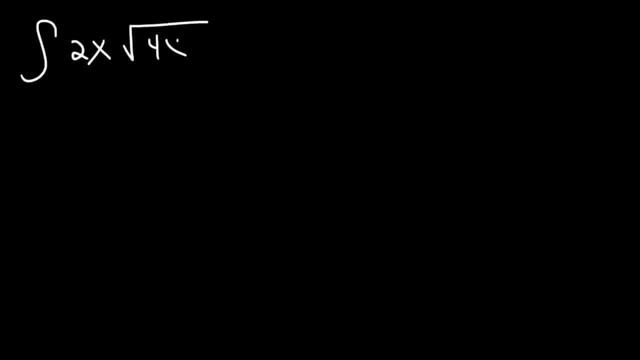 And that is it. Now let's work on this example. It's very similar to the last one, So you can try it if you want more practice. So let's set u equal to 4x minus 5.. Which means du is going to be the derivative of 4x. that's 4, and then times dx. 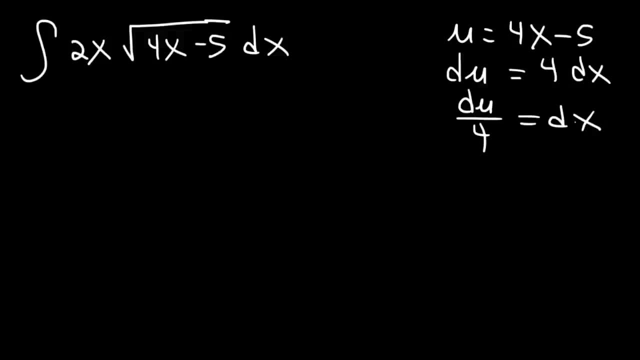 So solving for dx, it's du divided by 4.. Now we need to isolate x in this expression. So if we add 5, u plus 5 is equal to 4x, And then if we divide by 4, x is equal to this, which we can write it as 1 4th u plus 5.. 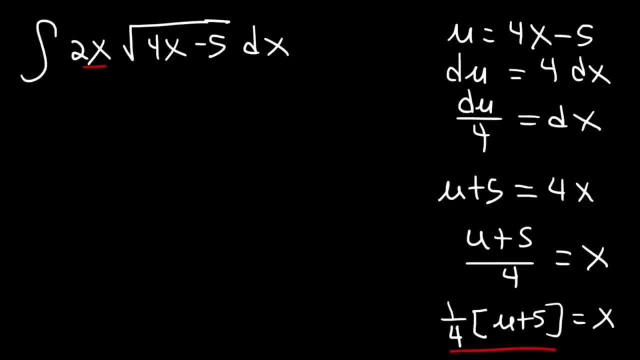 So let's replace x with this expression, and then 4x minus 5 with u, and then dx with du over 4.. So what we have is 2 times 4x 1, 4th u plus 5, and then the square root of u or u to the 1 half, and then dx is du over 4.. 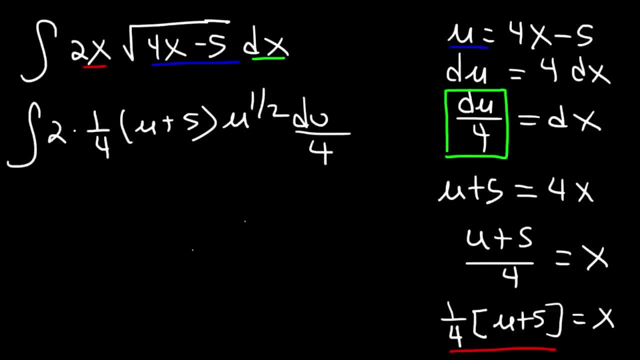 So 2 times 1, 4th is 1 half, and 1 half times 1 over 4 is 1, 8th. So we can move the 1: 8th to the front And then we have u to the half times u plus 5.. 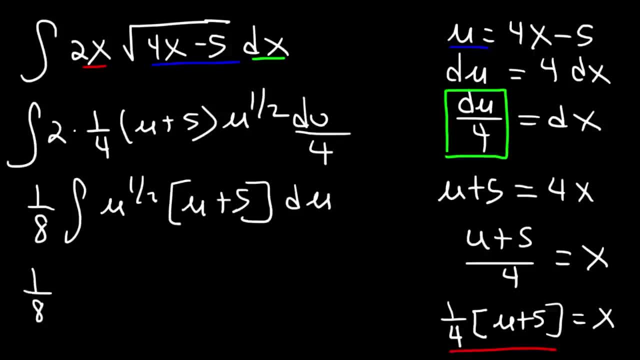 Now let's distribute: u to the 1 half, So u to the 1 half times u to the 1st power: 1 half plus 1, that's going to be 3 over 2.. And then plus 5, u to the 1 half. 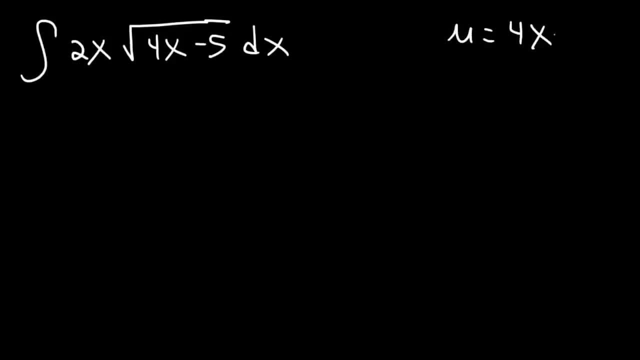 so let's set you equal to 4x minus 5, which means du is going to be the derivative of 4x, that's 4, and then times dx. so solving for dx its du divided by 4. now we need to isolate x in this expression. so if we add 5, u plus 5 is 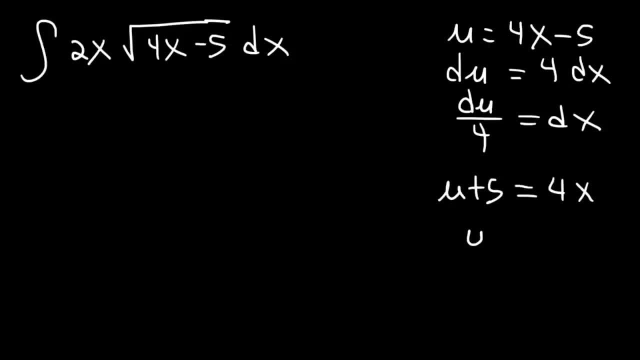 equal to 4x, and then, if we divided by 4, x is equal to this, which we can write it as 1 fourth u plus 5. so let's replace x with this expression, and then 4x minus 5 with u, and then dx with du over 4, so what we have is 2 times. 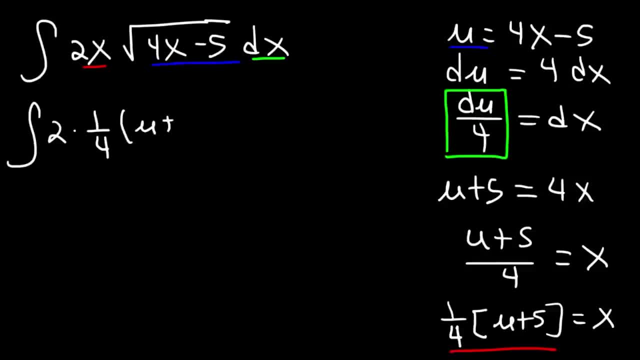 1, fourth u plus 5, and then the square root of u or u to the 1 half, and then dx is du over 4. so 2 times 1 fourth is 1 half, and 1 half times 1 over 4 is 1. 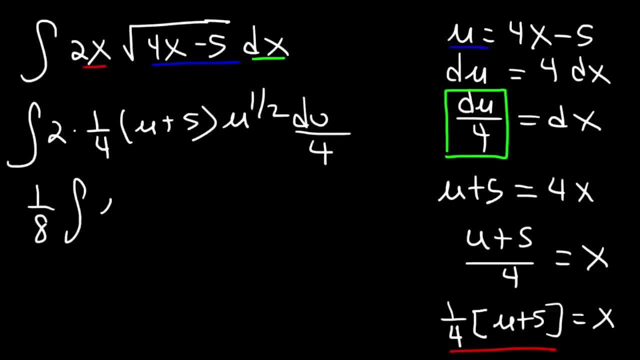 eighth, so we can move the 1 eighth to the front, and then we have u to the half times u plus 5. now let's distribute u to the 1 half, so u to the 1 half times u to the 1st power. 1 half plus 1. that's going to be: 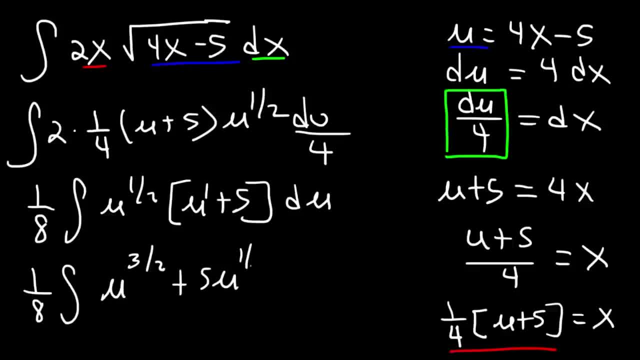 3 over 2 and then plus 5 u to the 1 half. so now we need to integrate the expression that we now have. so this is going to be 1 over 8 u, 3 over 2 plus 1, that's 5 over 2, and then. 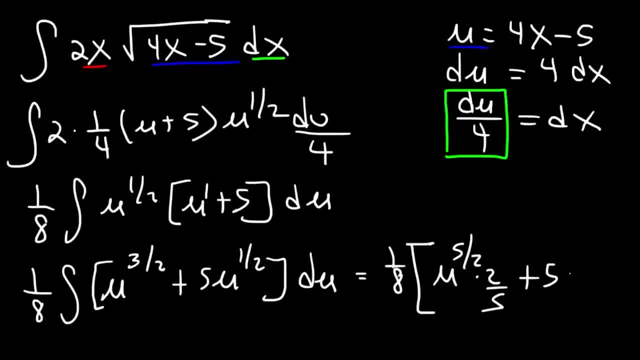 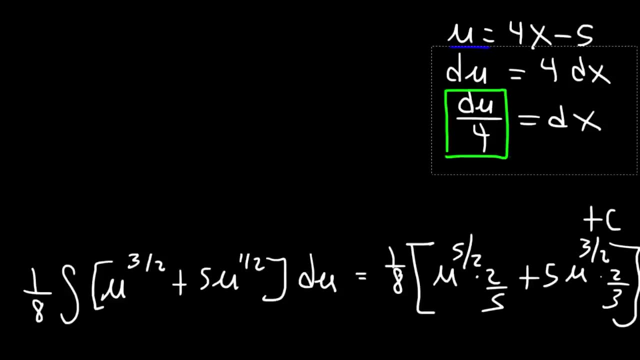 times 2 over 5, and then 1 half plus 1 is 3 over 2, times 2 over 3, and then plus c, 1 over 8, times 2 over 5, that's going to be 2 over 40, and then times u raised to the 5 over 2, and then